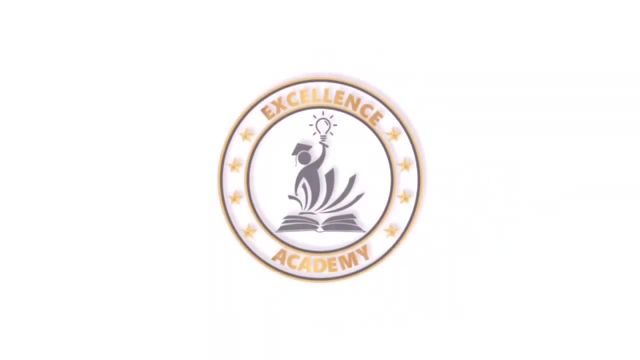 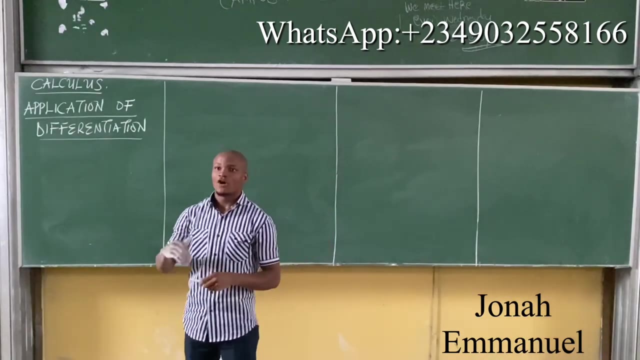 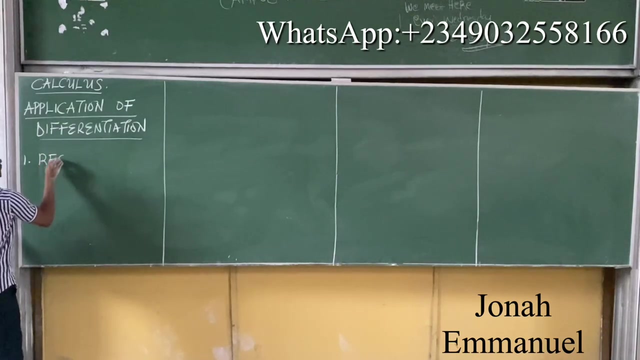 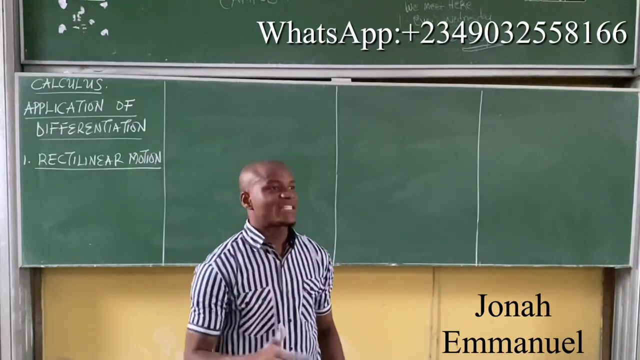 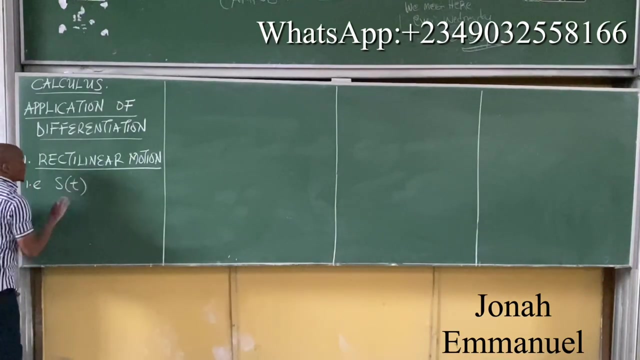 So let's look at the application of differentiation. The various applications of differentiation include number one: rectilinear motion. Rectilinear motion Given distance, slash displacement. Given distance or displacement as a function of time. That is, that is s of t, Given distance or displacement as a function of time. 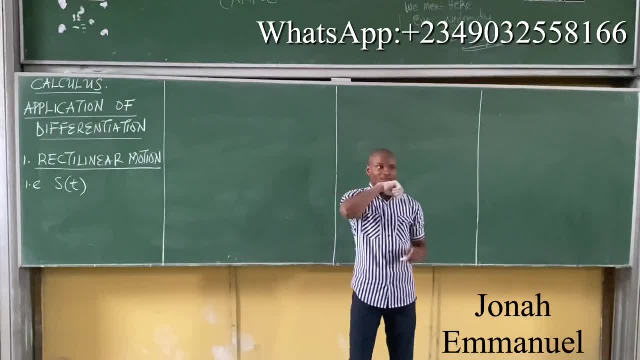 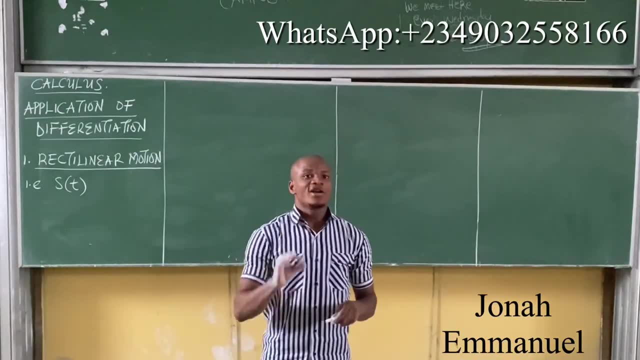 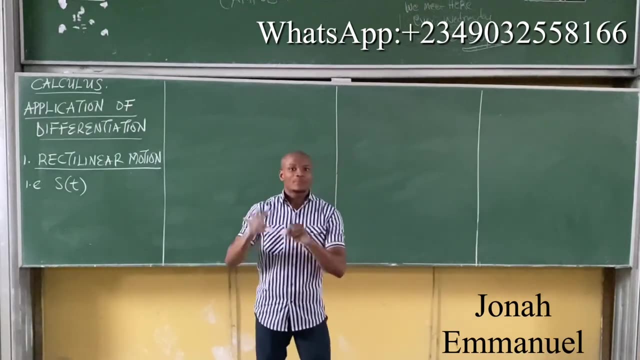 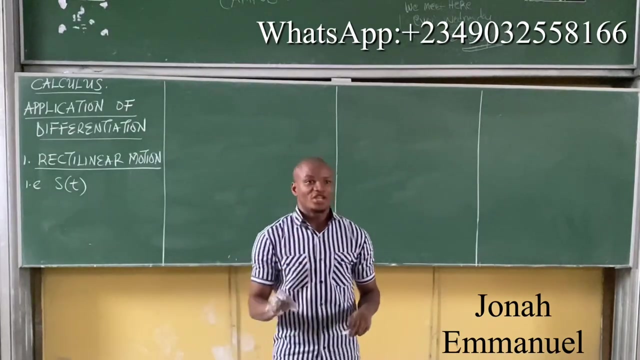 That is the s over the t. Recall that velocity or speed. Recall that velocity or speed Is the rate of change. recall that velocity or speed is the rate of change of displacement or distance respectively. Is the rate of change of displacement or distance respectively. 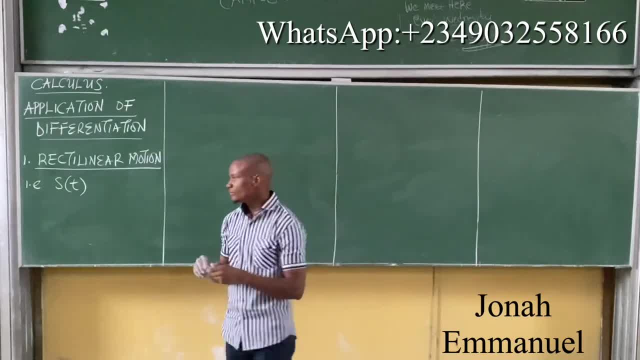 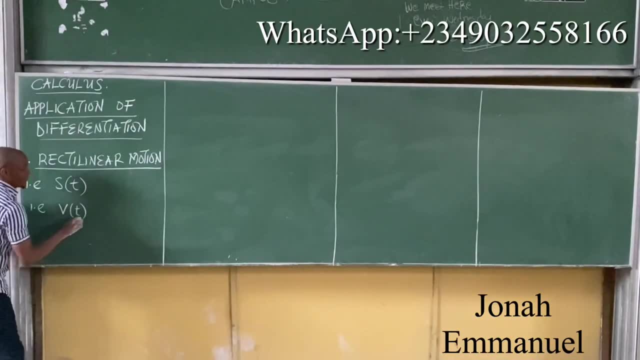 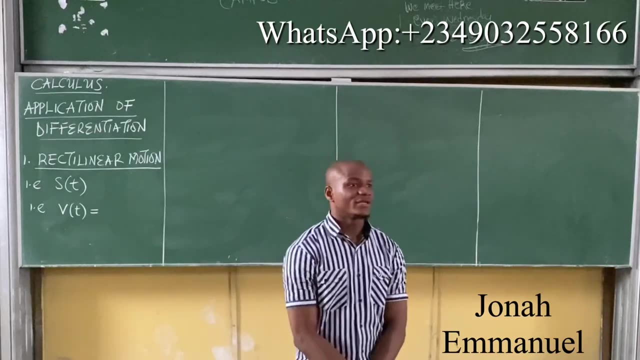 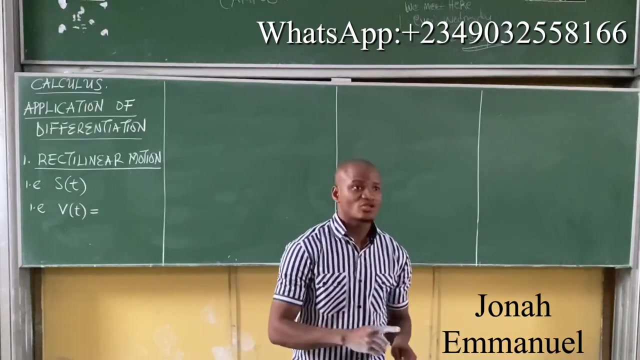 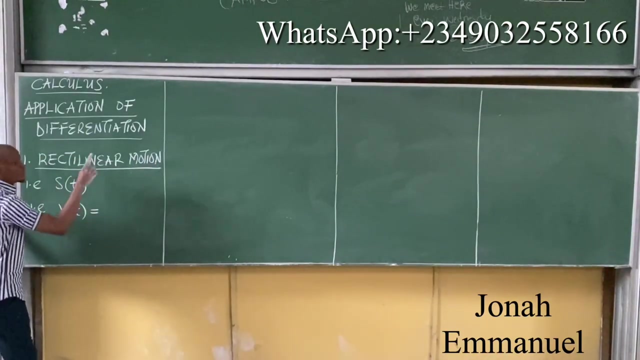 That is the rate of change of displacement or distance. That is. we're saying that velocity expressed in terms of time is the rate of change of displacement. Please don't always say rate of change. What does it mean? What does it mean? It means a parameter is what Changing with respect to time? And if we say displacement is x, change displacement with respect to time, it becomes what there ds, over what dt. So I have this: 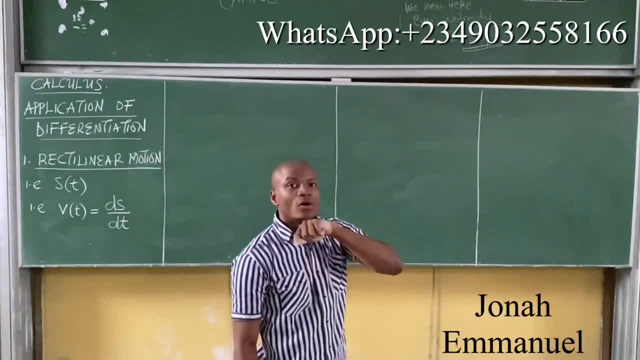 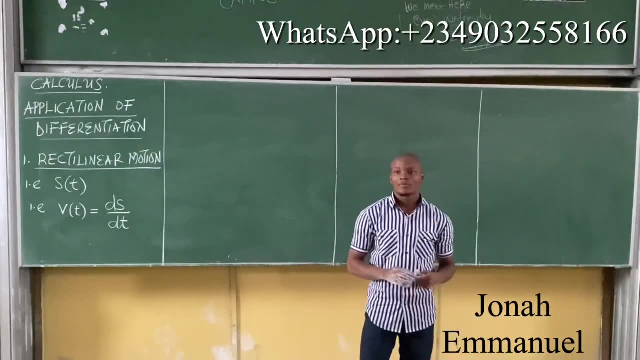 Alright, Also recall that, if you're here. so I say that v of t is equal to ds of t. Alright, Also recall that, if you're here. so I say that v of t is equal to ds of t. So I say that v of t is equal to ds of t. 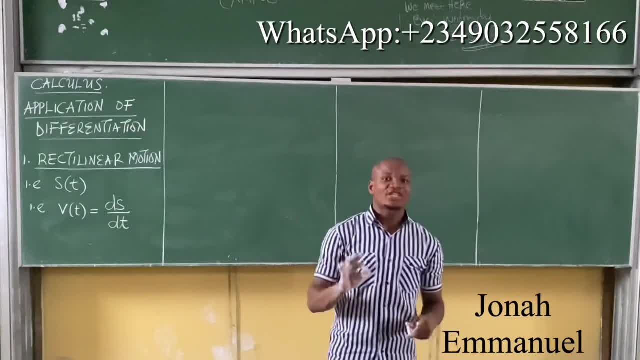 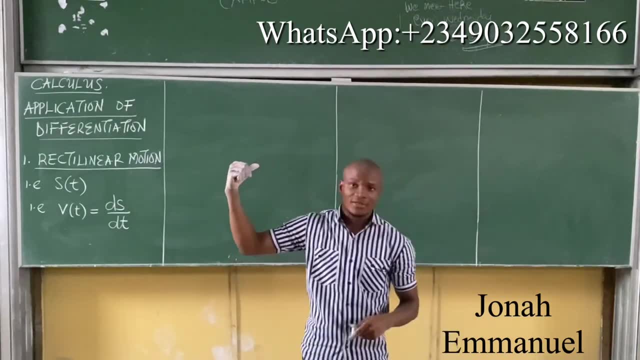 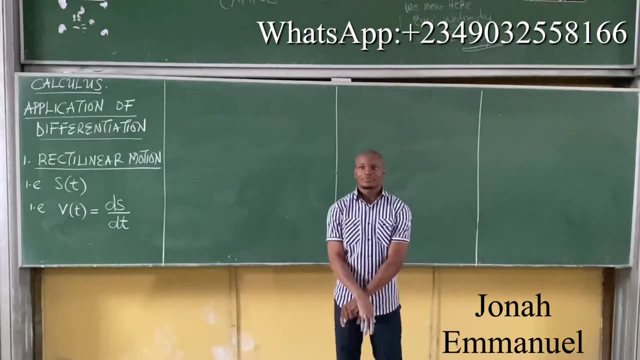 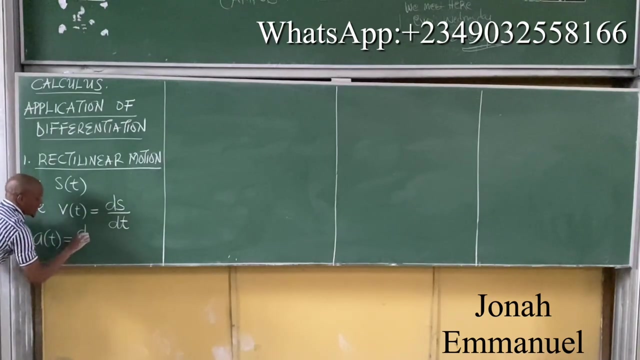 Alright, Also recall that acceleration is the rate of change of velocity. These concepts are from physics, You should notice. Alright, Also recall that acceleration is the rate of change of velocity. So you are saying that a of t acceleration is equal to dv all over the t is equal to. 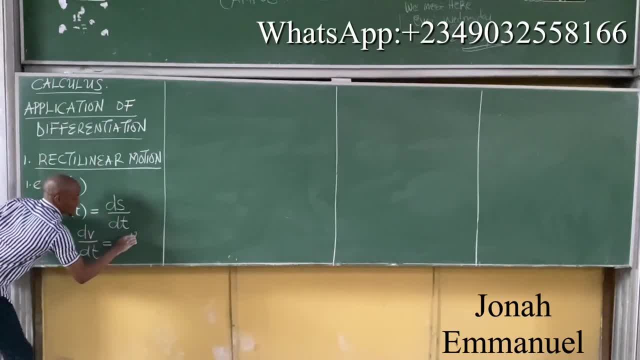 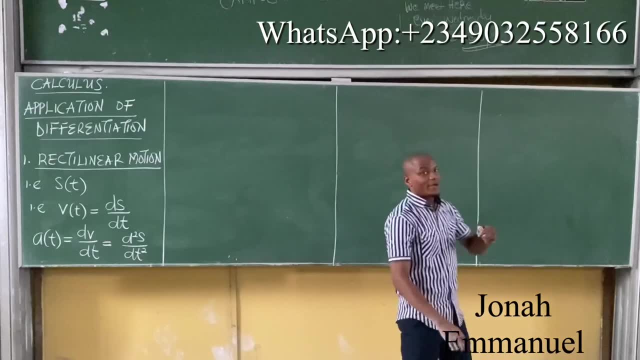 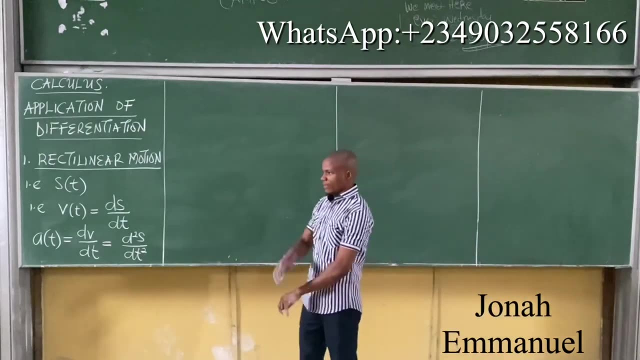 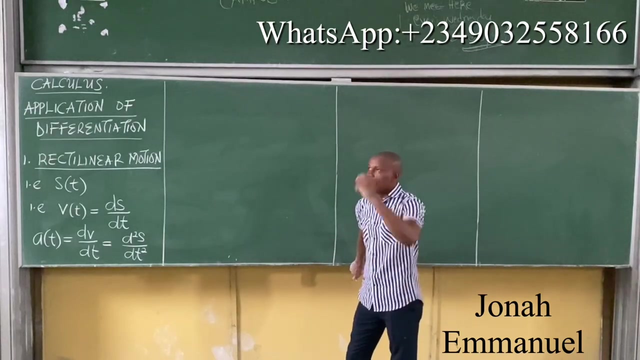 In terms of distance, we call it dv over the t. Yeah, Cos d squared x all over d t squared. Cos d squared x all over d t squared. Cos d squared x all over d t squared. What does this mean? Before this, let me show you this proof. 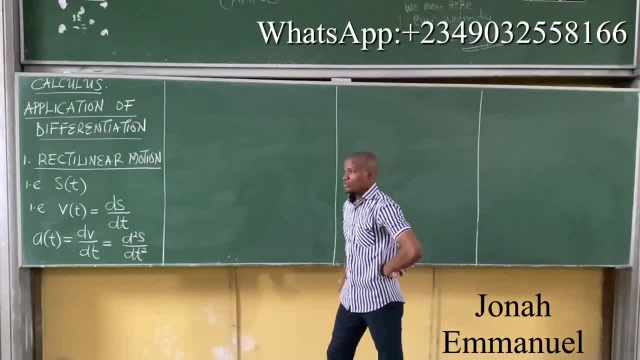 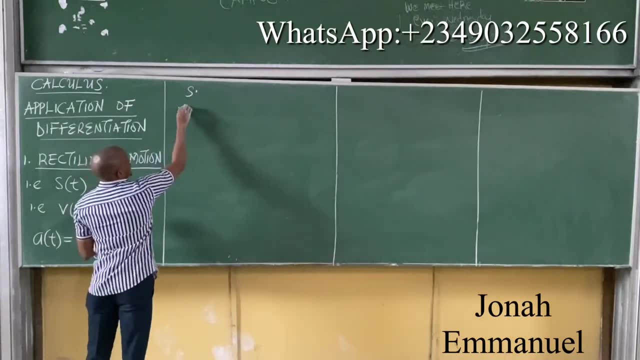 Look at this Before this. let me show you this quickly, please. So here's the concept. I have distance S. Velocity V is equal to, we said, rate of change of distance or displacement. In this case I used interchangeably. 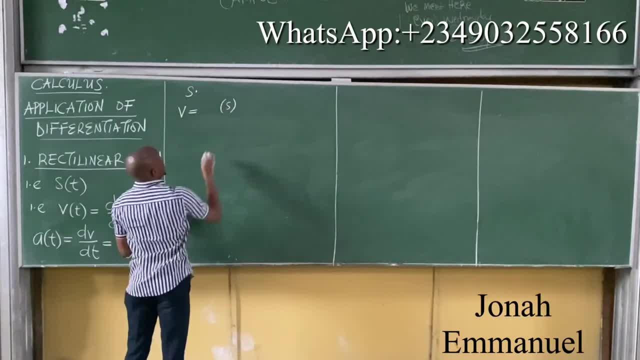 So when we say rate of change, it means that the S is changing with respect to time. So we call Z over the T of S point above. So V is equal to Z over the T of S. That means changing with respect to time. 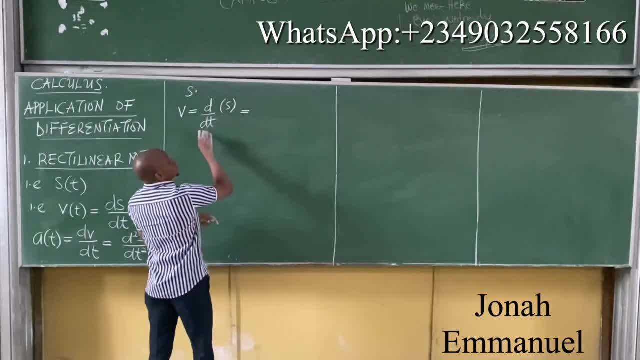 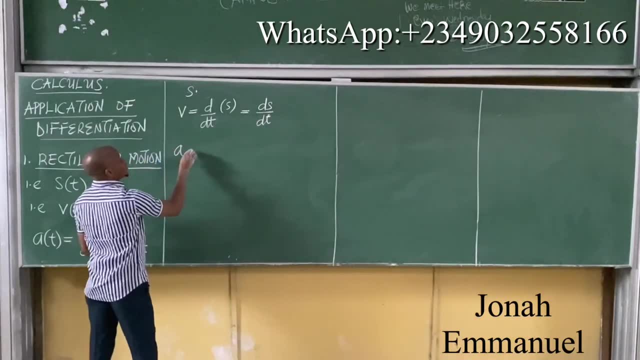 of distance or displacement. If I multiply these two, this and this, this means the S all over Z. That's one. Next up, we said acceleration is rate of change of velocity, So hence it becomes Z over the T, Changing with respect to time. of which parameter? 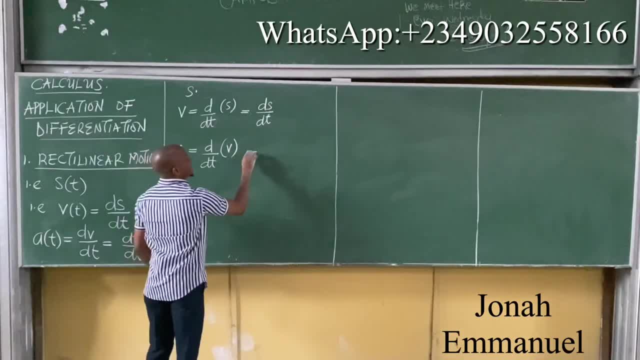 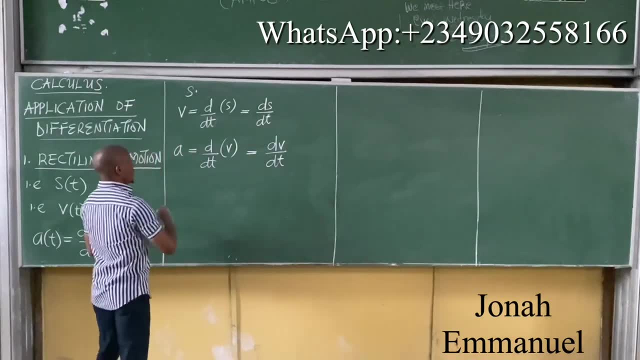 we said velocity, so harvest. So if I multiply this and it becomes D times V, gives you the V all over to the T, But again we can see that A is equal to this D all over the T of V. From here we said V is equal to the S over the T. 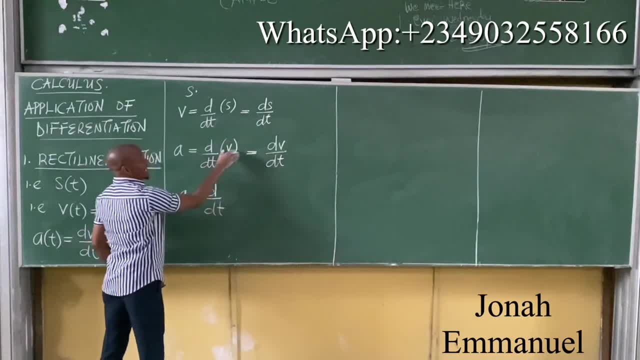 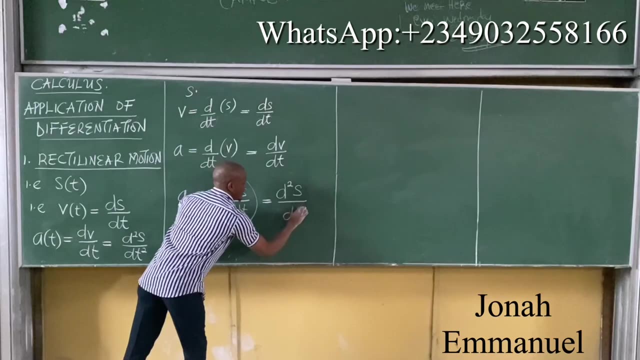 So I can replace V here by the S over the T. Take out this math and put the S over the T in strength. This will be equal to: Z times Z gives you the squared S all over the T times T gives you the T squared. 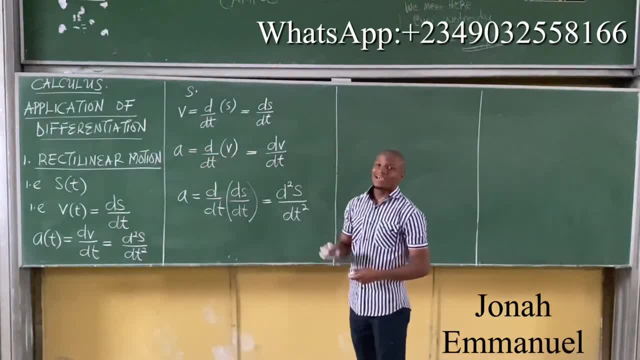 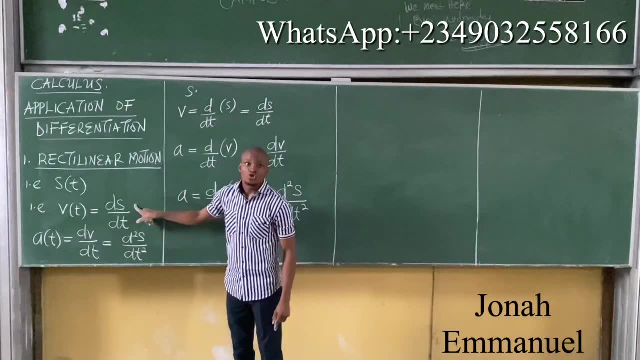 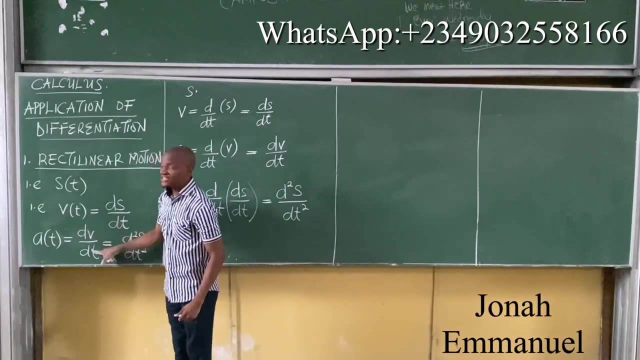 That's how we got this measure. That's the idea. So the idea here is very simple. If I'm given distance to get velocity differentiate once, To get acceleration differentiate twice, that's all. If I'm given velocity to get acceleration, 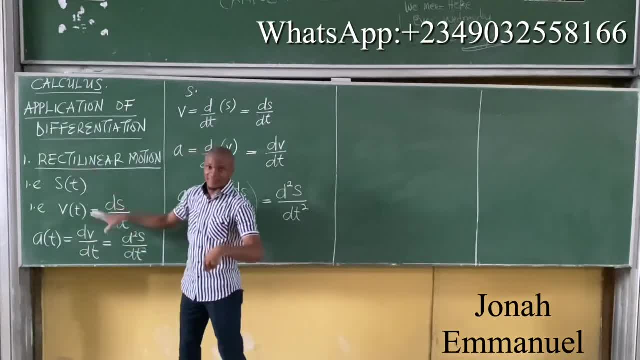 which number times there? Just once. So please notice this thing: If I'm given distance to get velocity differentiate once, From distance to acceleration differentiate twice, But if I'm given velocity, of course, for me to get acceleration differentiate just once. 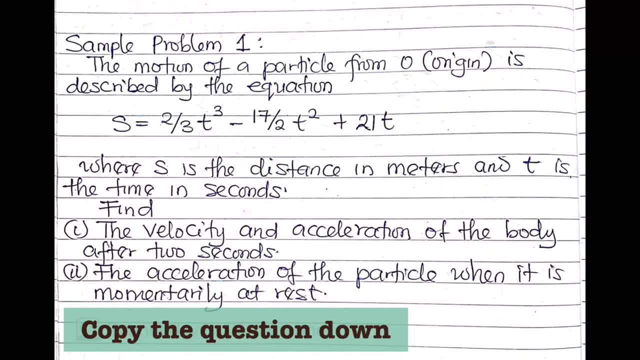 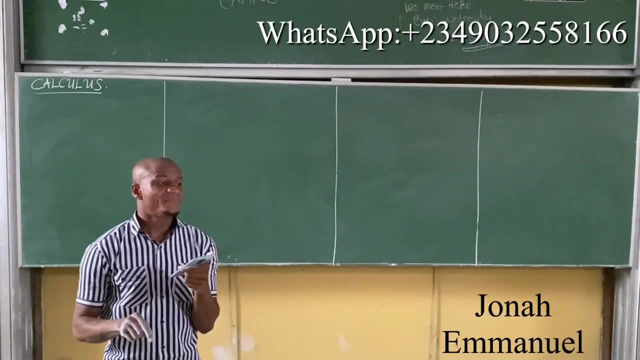 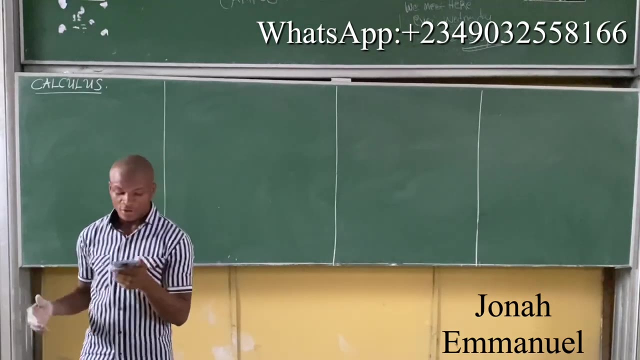 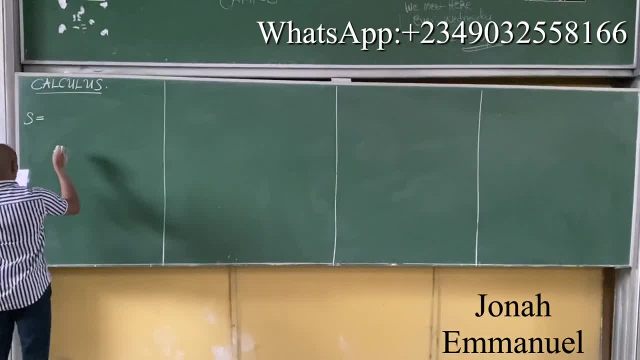 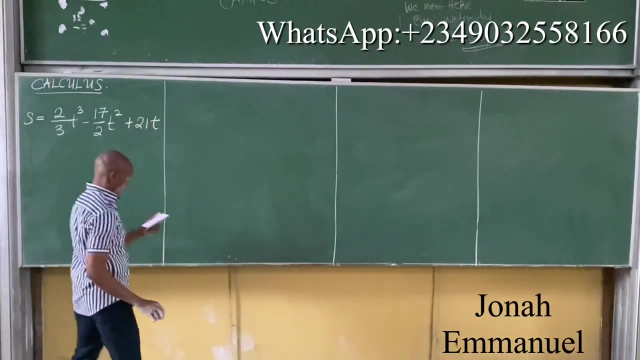 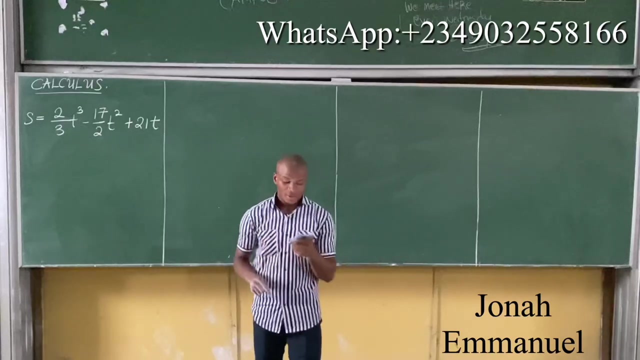 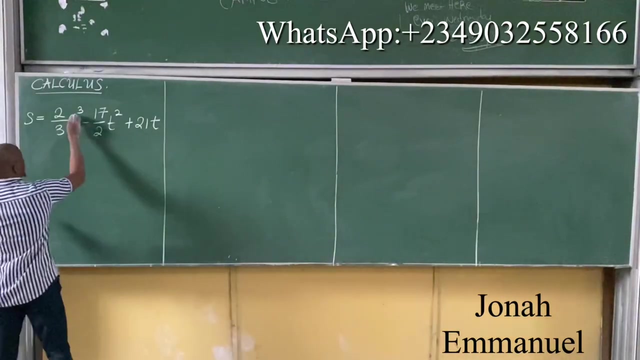 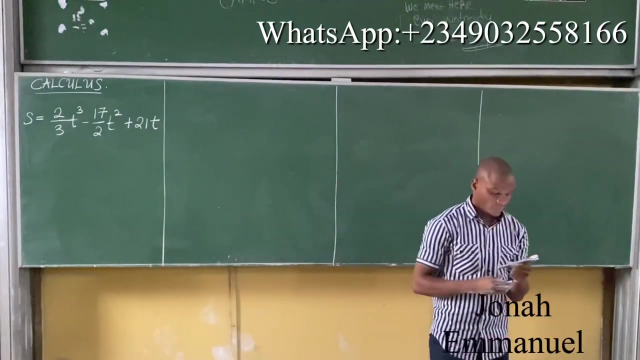 Is described by the equation X, is equal to 2 over 3 T cubed minus 17 over 2 T squared plus 21 T. The motion of a particle From O- I said O there represents origin- Is described by the equation X equal to 2 over 3 T cubed minus 17 over 2 T squared plus 21 T. 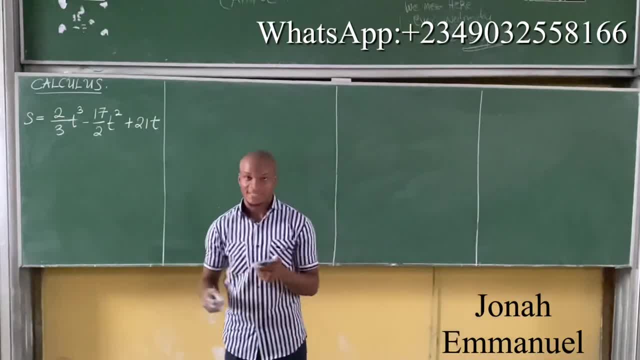 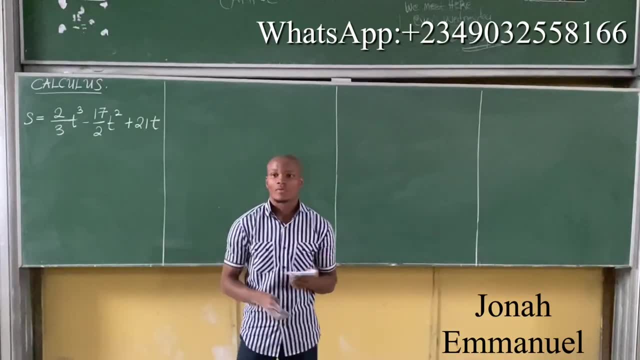 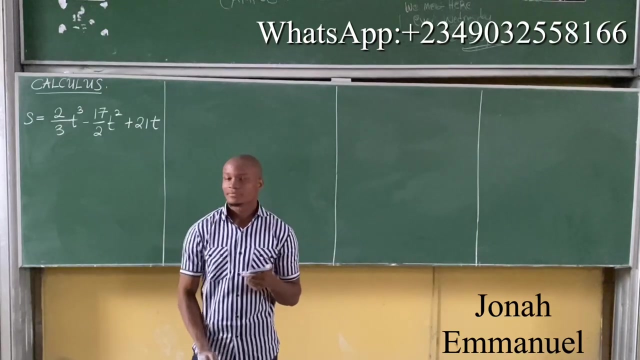 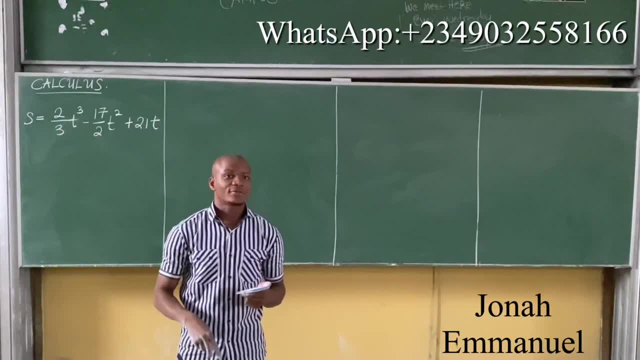 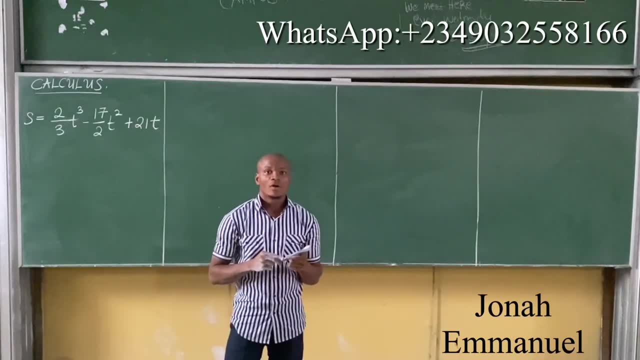 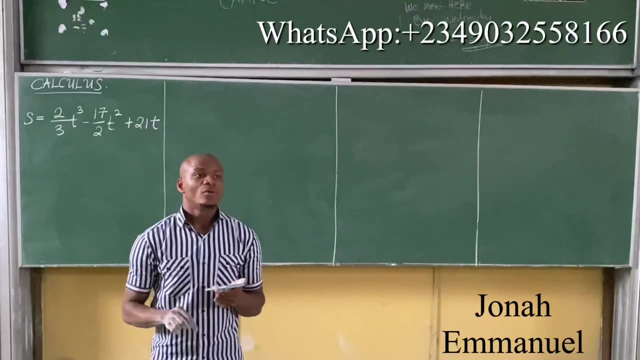 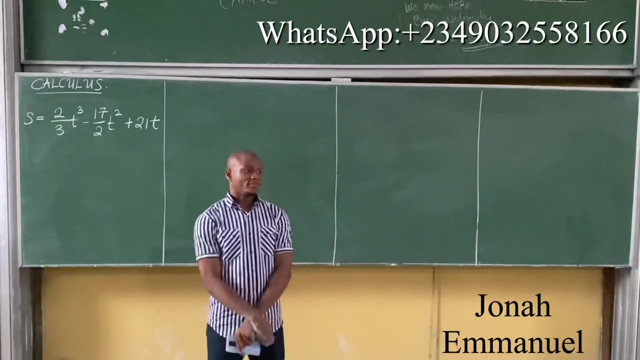 after two seconds I find the acceleration of the particle. find the acceleration of the particle after two seconds when it is momentarily at rest. alright, let's get this done. what's the iPad is after what there? so they say: find velocity and acceleration after two seconds. 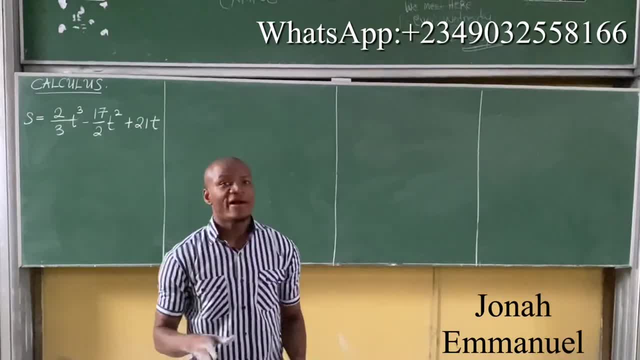 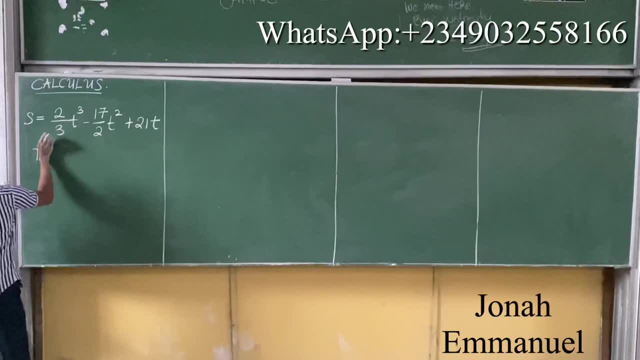 your first case would be: find the velocity equation, find the velocity equation, find the velocity equation. so from here, take a look at this: the velocity equation, the velocity equation will be, will be. we said b is equal to the s over 3, so I have that b is equal to. 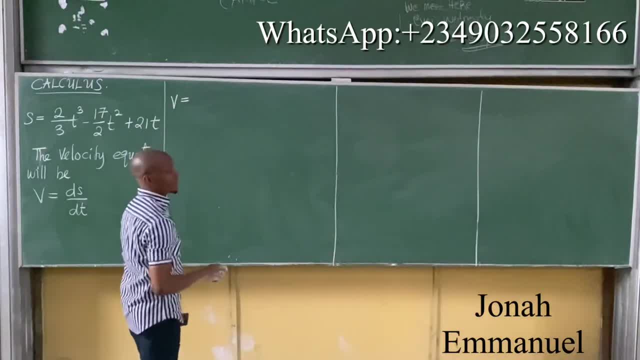 now, look at this, look at this, just for writing sake. look at this. it means I am differentiating this one here, we know, but just for writing sake, please, it's better you express this way, express it as d over the t of x. that's this. 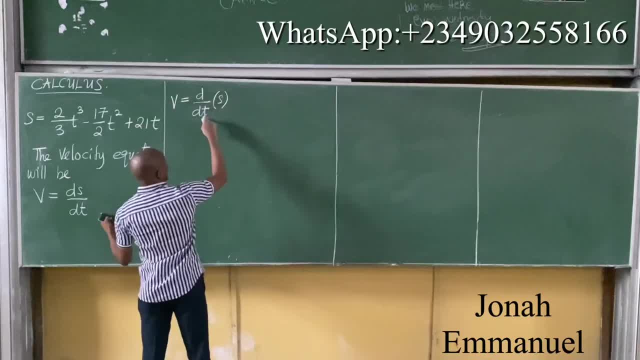 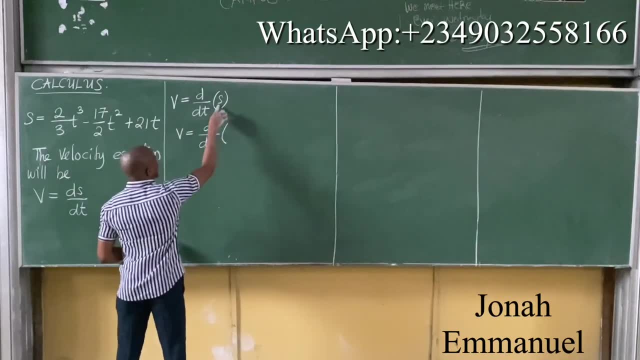 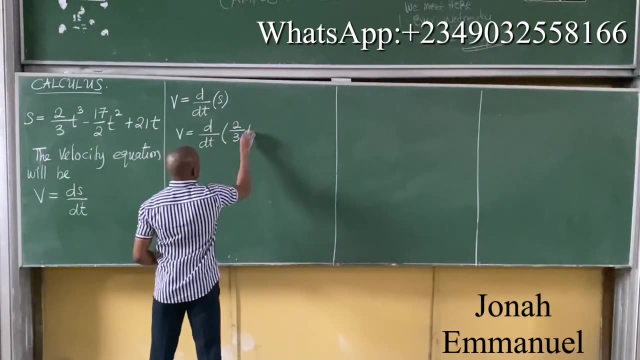 d over the t of x. the same thing there, the s over the t and that's equal to. so b is equal to d over the t of x. what's x? this equation? so bring this equation here. it becomes 2 over 3 t cubed. 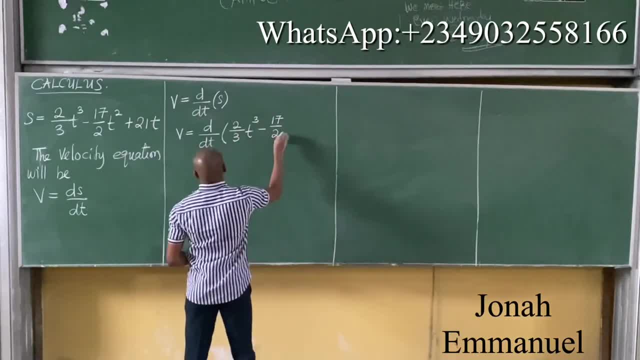 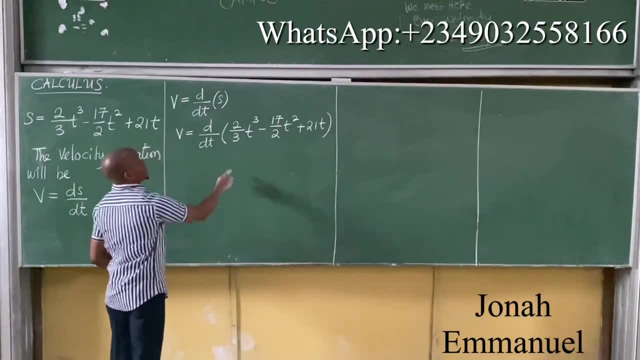 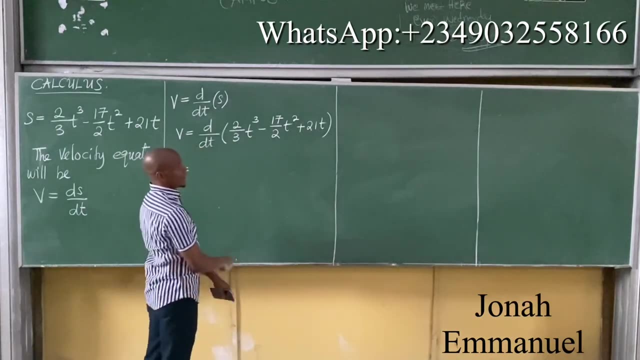 minus 17 over 2 c squared plus 21 t. so I am simply differentiating. this. that means b is equal to, that means b is equal to. please for this one. which method do I use here? general method, have you right? so we said. 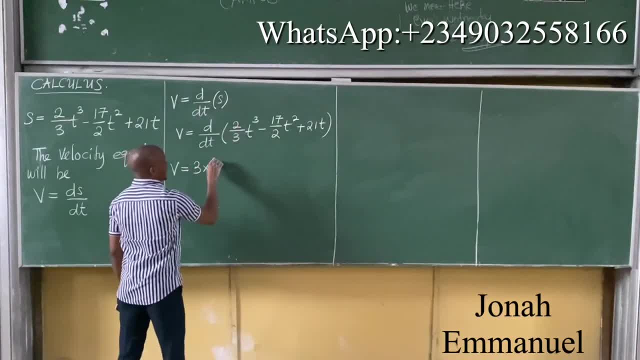 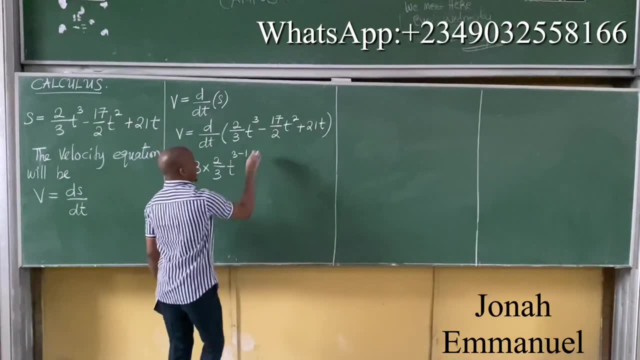 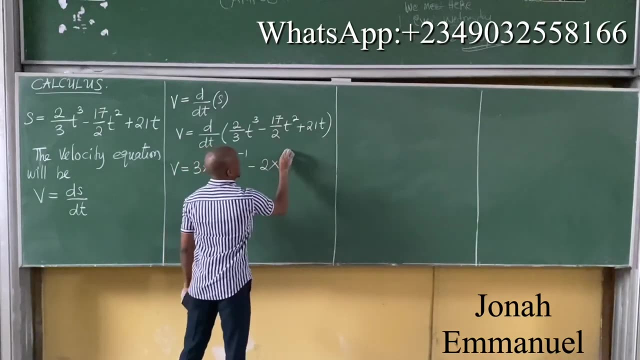 multiplied by the power, becomes 3 times. what I do is what I have here: 2 over 3 t. subtract 1: 3 minus 1 minus same thing here, multiplied by the power: 2 times what I have here: 17 over 2 t. 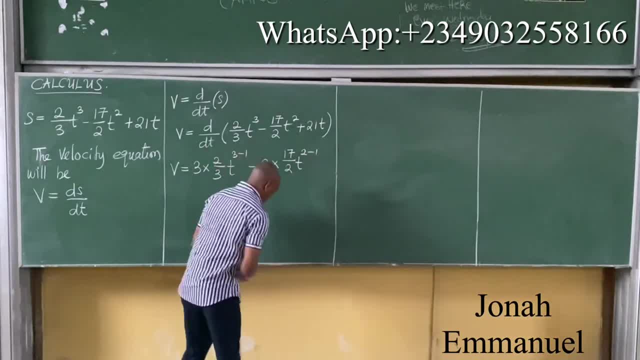 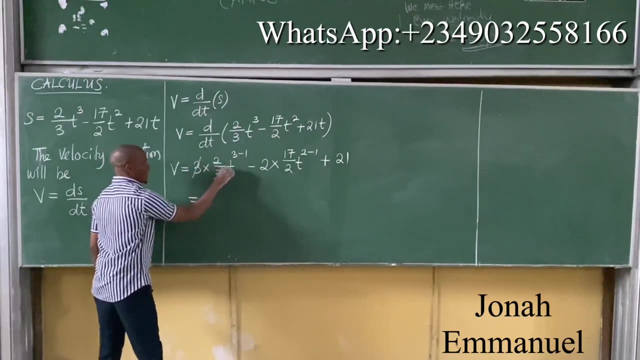 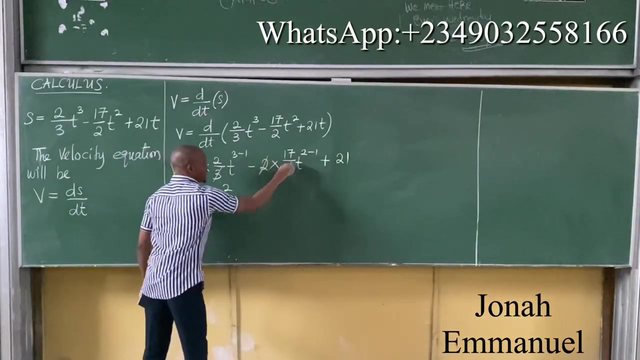 subtract 1, 2 minus 1 plus differentiating 1 t. what do you get here? it is 21, so I have this. work this out. this will cancel this. what do I get? 2 t squared 3 minus 1 minus. this can cancel this. 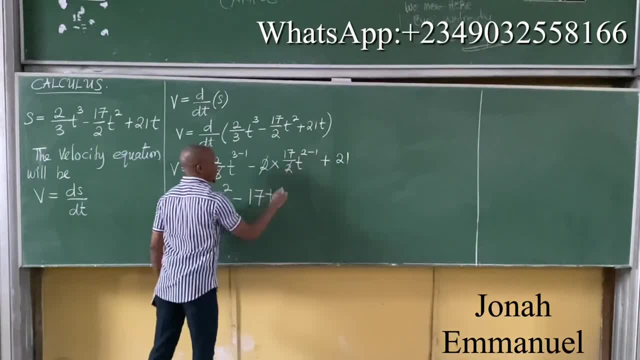 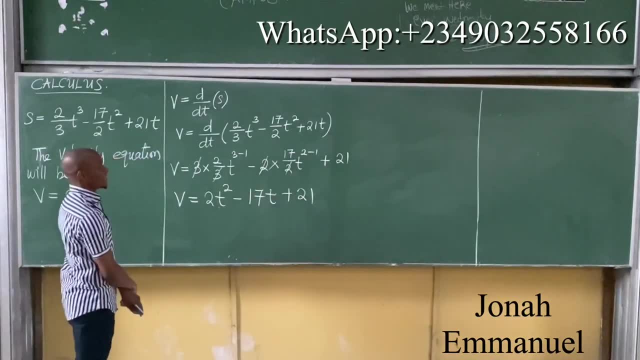 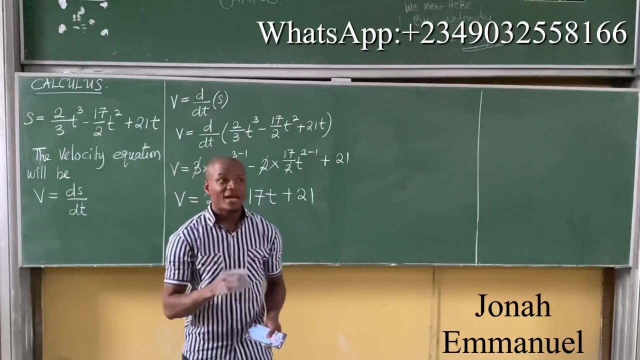 what do I get? 17 t 2 minus 1 is 1 plus 21. this is the velocity equation. next task: get acceleration equation because we have to find velocity and acceleration. after 2 seconds I have gotten velocity. we said to get acceleration, simply differentiate. 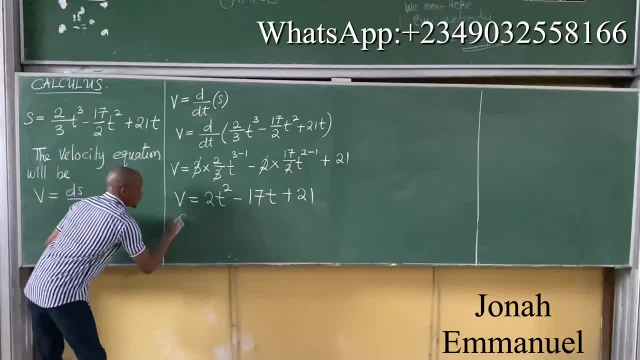 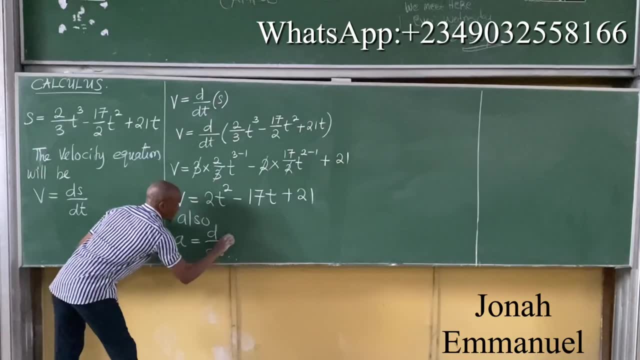 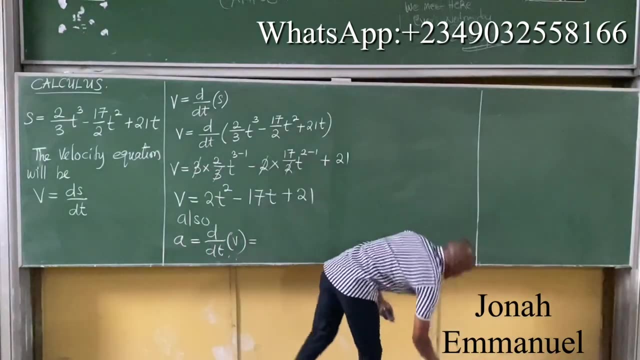 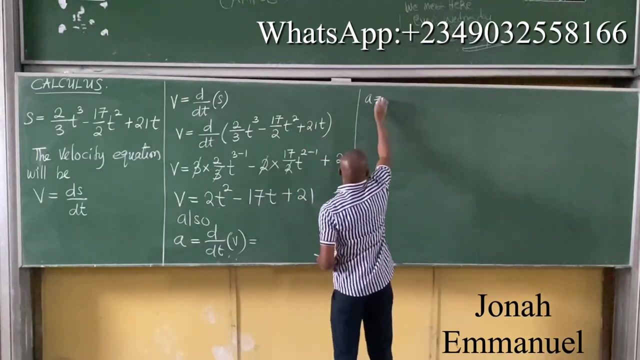 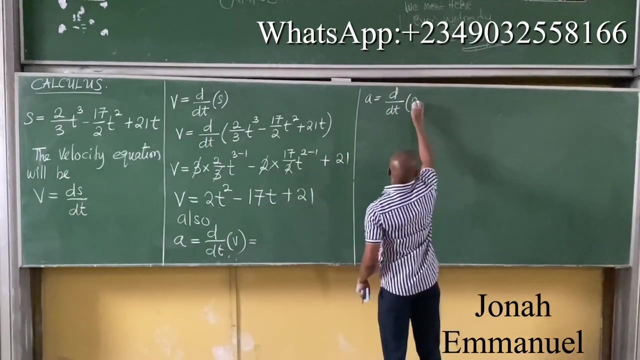 water velocity. so also we know that acceleration a is equal to water, d over the t of v, and that's equal to, and that's equal to d all over the t of what's v. all of this, that becomes 2 t squared minus 17 t. 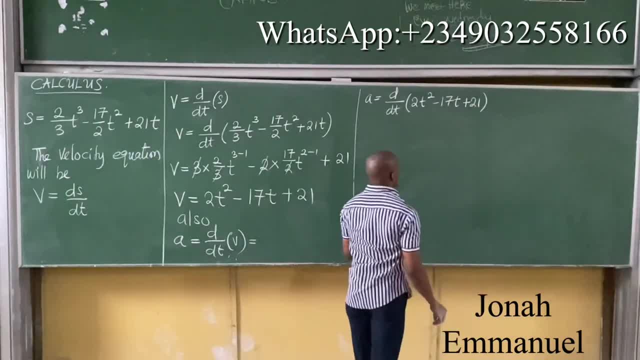 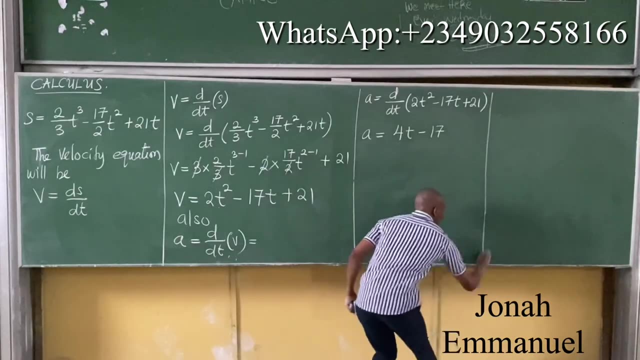 plus 21, of course, differentiating. so we have that a is equal to over here this and this: 40 minus 17, plus what there, 24, 24. so with this one there I've gotten velocity equation and acceleration. now say: find velocity and acceleration. 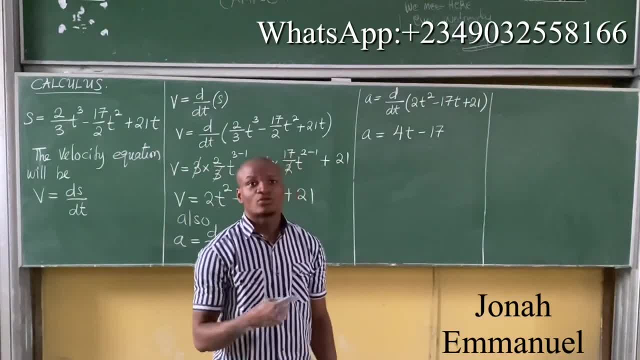 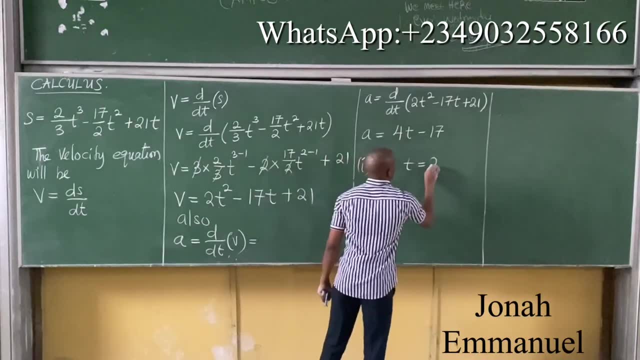 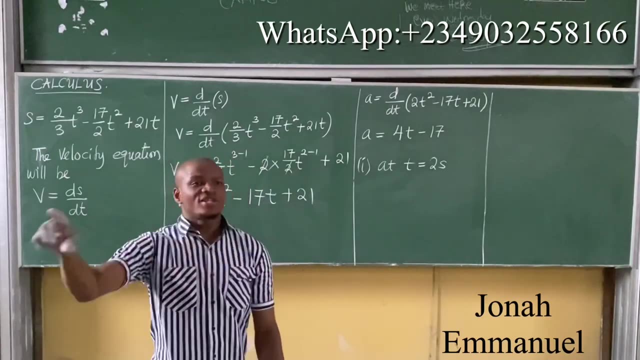 at t equal to 2 seconds, so i i at t equal to 2 seconds, so I find it after 2 seconds, so I find it after 2 seconds. here's where the problem comes in. here's where the problem comes in when you read the question. 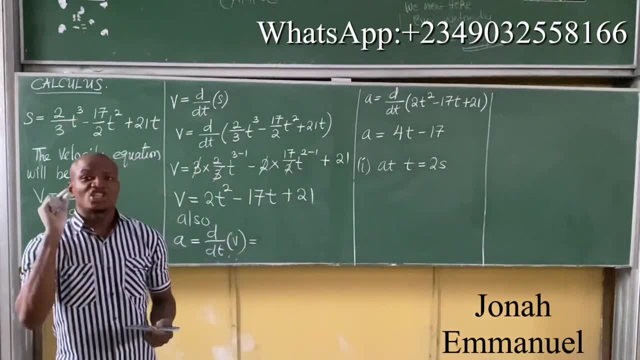 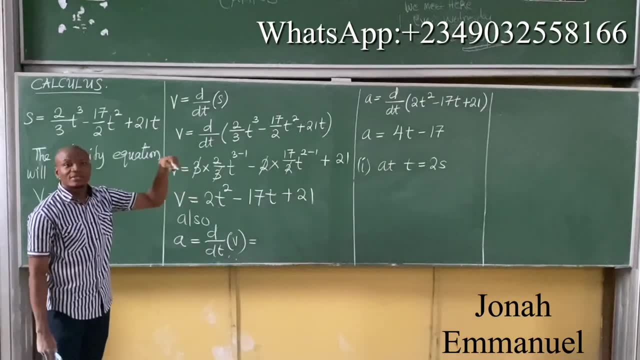 when you read the question, try to grasp what they are saying. now observe. they define each text. they say: ys is what they say. ys is what. distance in meters. distance in meters and t is what there and t is what there. time in what? 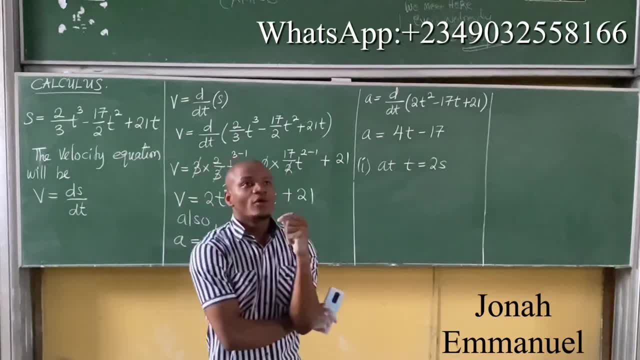 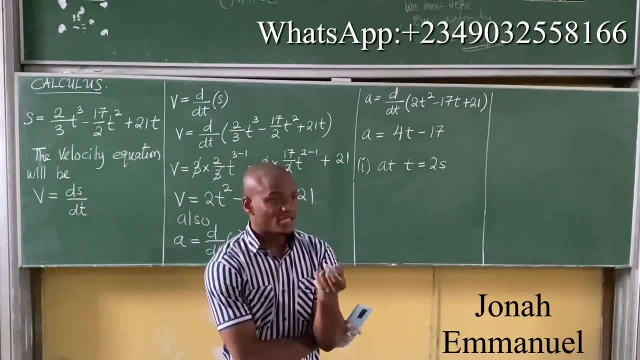 seconds. so here's the indication now. so here's the indication now. what did they say? find the velocity and and acceleration of the body after, after 30 minutes, after 30 minutes, after 30 minutes. what do you do the best? convert, convert the second first. 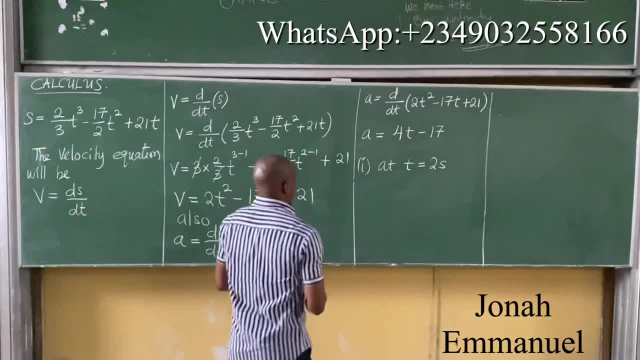 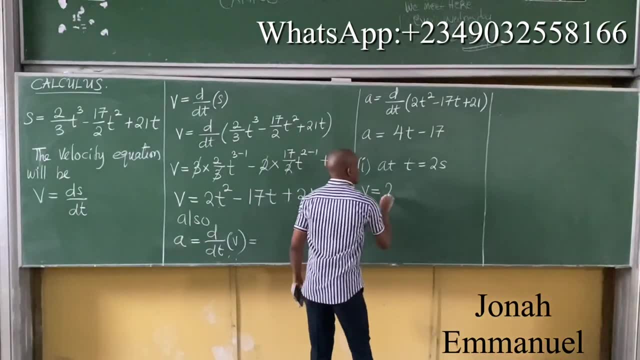 convert the second first, before it's altitude, before it's altitude, alright, at t equal to 2 seconds. we have that velocity is equal to this. velocity is equal to this: 2t squared, 2t squared minus 17t, minus 17t plus 21. 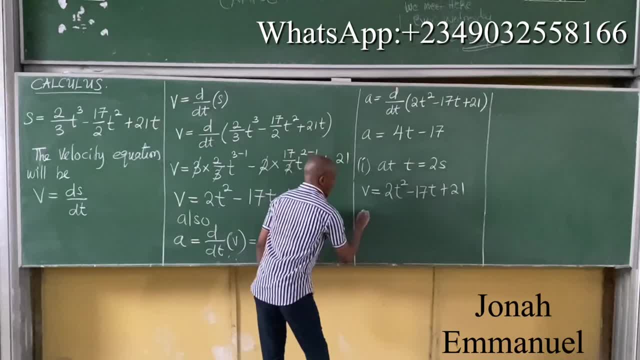 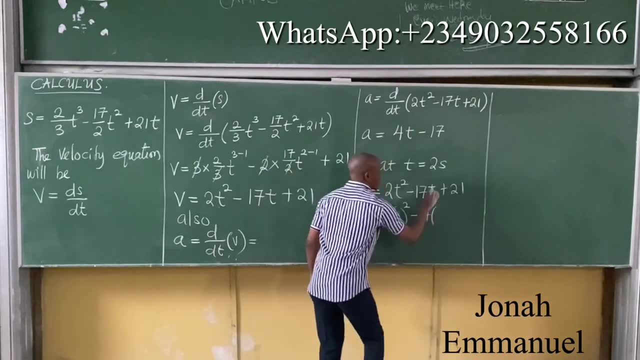 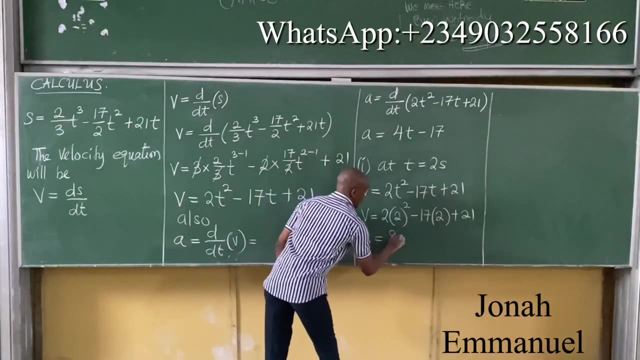 plus 21. so put t here. so put t here as 2. we have that v is equal to 2 into 2. squared minus 17 into 2 plus plus plus 21, this is equal. to this is 4 times 2, that's 8. 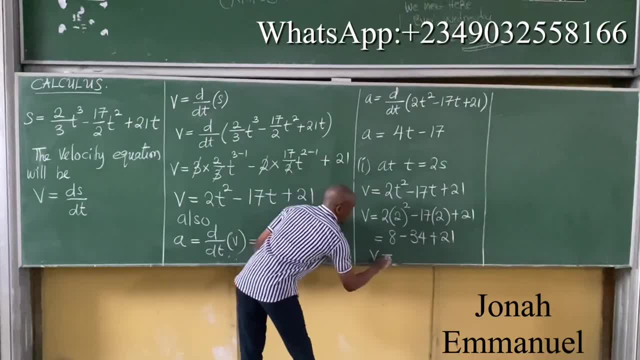 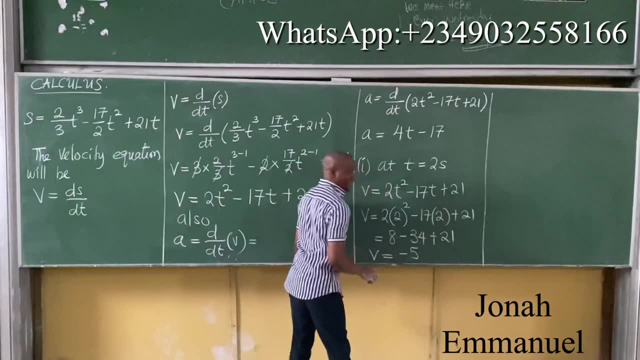 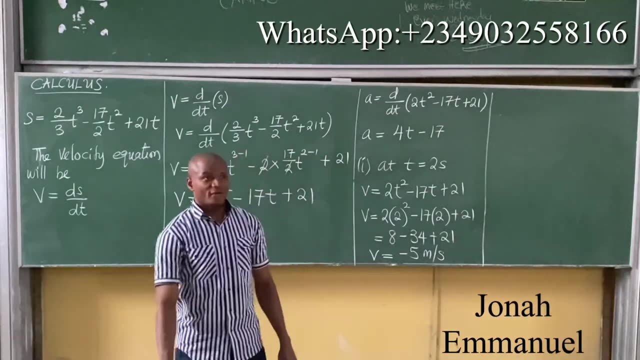 minus this and this, that's 34 plus 21, so v is equal to what do you have here? sorry, sorry, minus 5 minus 5. minus 5 units. units per second per second per second. meters per second. meters per second. please also put unit, please. 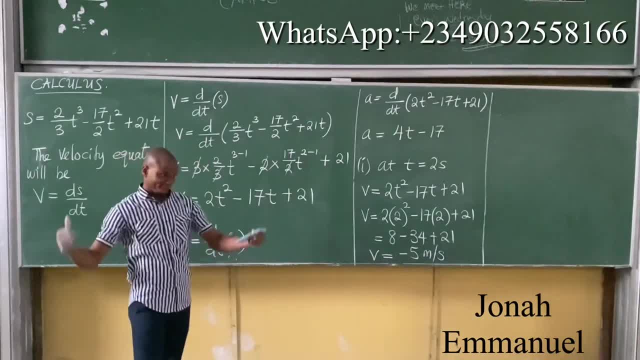 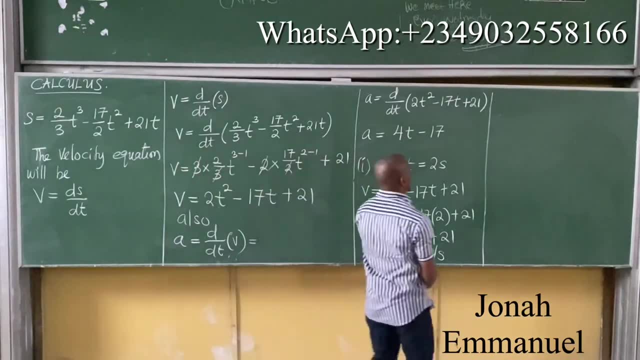 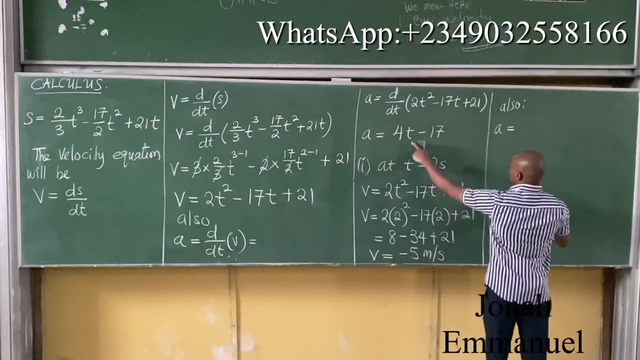 please also put unit please. it's minus 5, so the car is going back. it's going back negative 5, alright meters per second. next up they said acceleration also. we have that. acceleration is equal to your equation is 4 t minus 17 and that's. 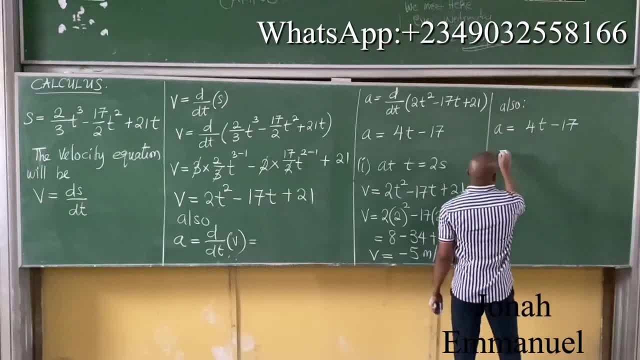 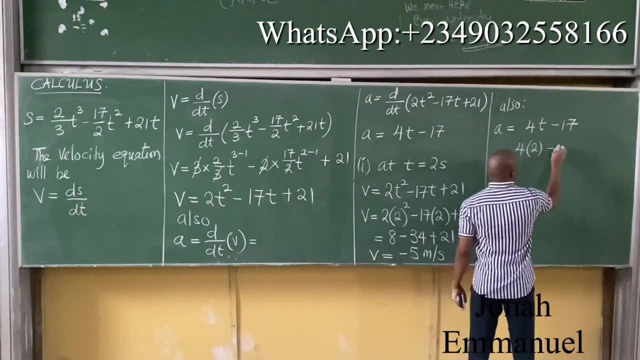 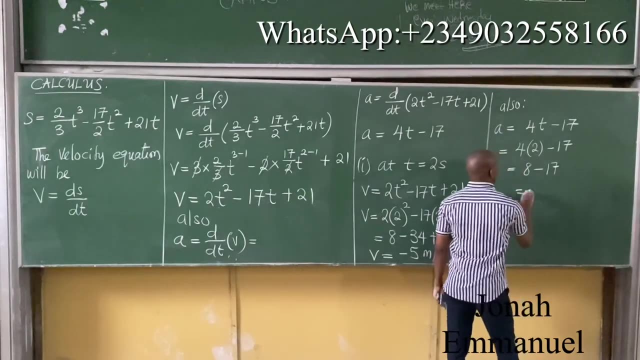 equal to 4. we said at 2 seconds becomes this: this must become 2 minus 17 minus 17, that's equal to 4 times 2 is 8 minus 17. 8 minus 17 minus 11 minus 9, please units. 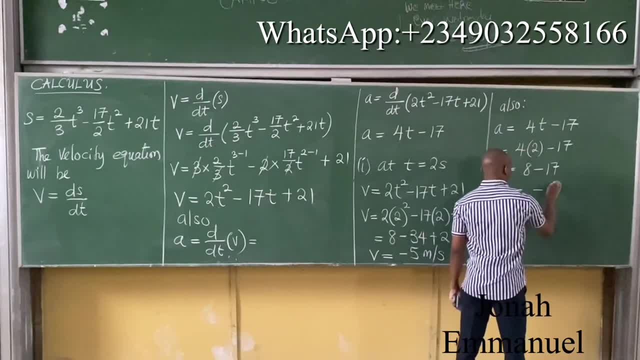 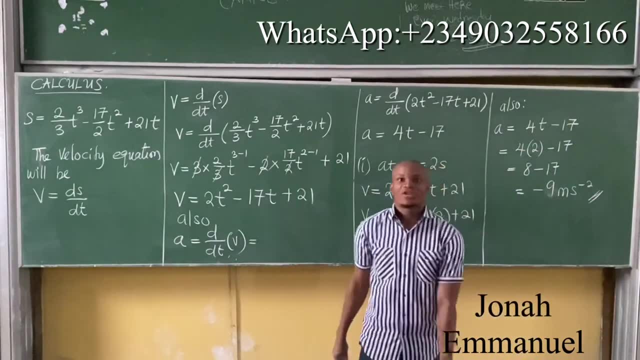 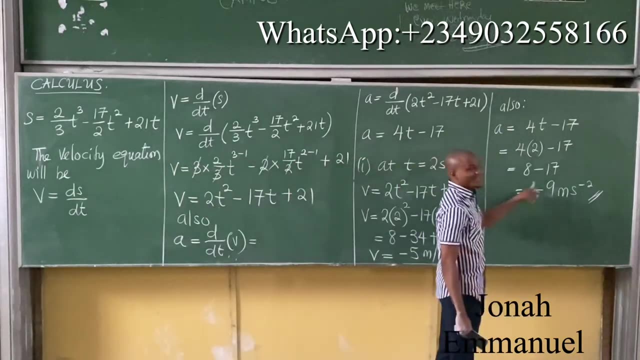 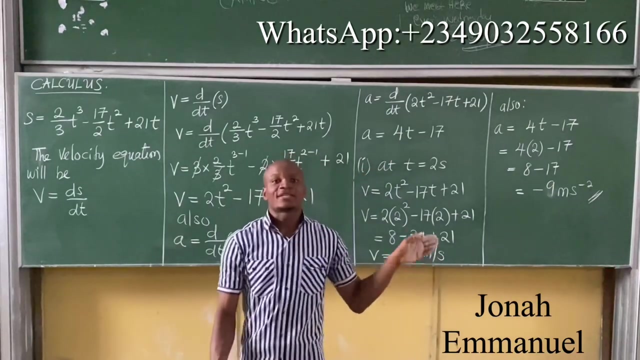 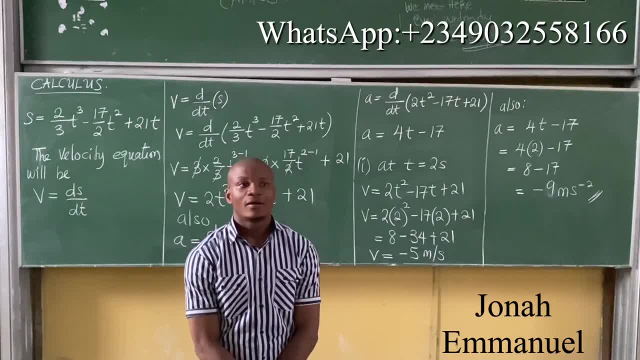 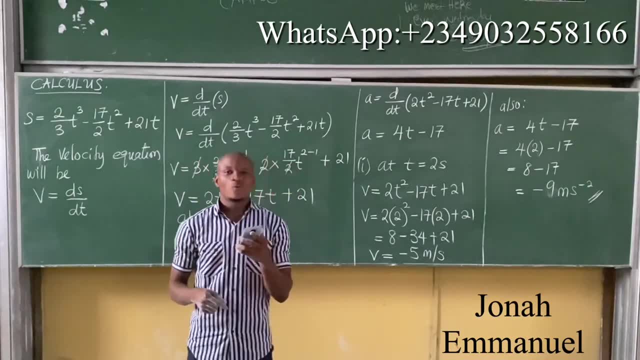 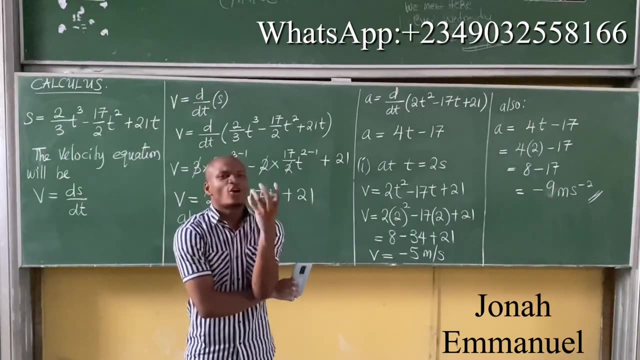 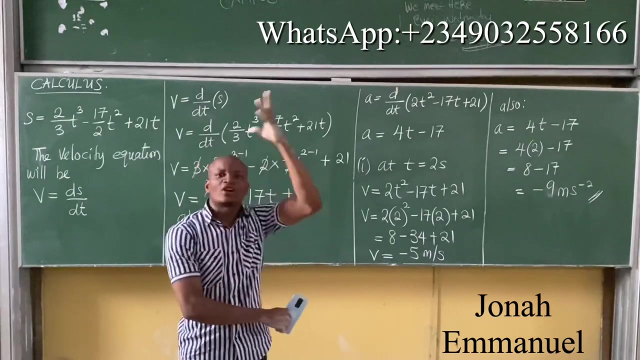 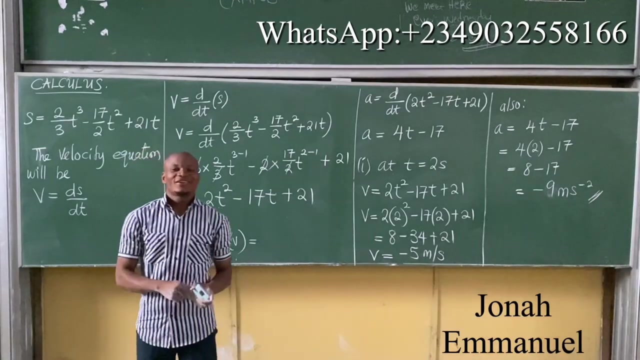 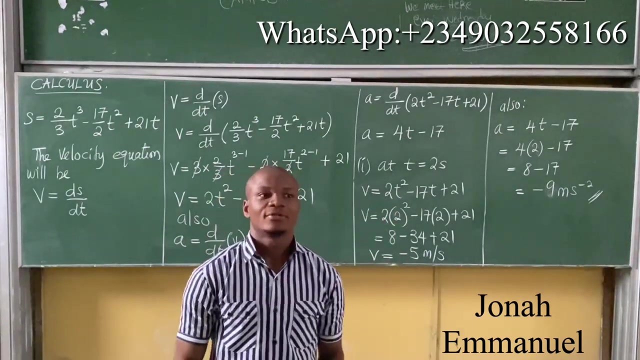 6 steps, please. alright, let's take me to do this. what we are actually doing, that even this, yes, still lead- are I get when a body is at rest, what the condition died in it? when it's in the finger finger, when a body is at rest, its velocity cell? that's a condition that 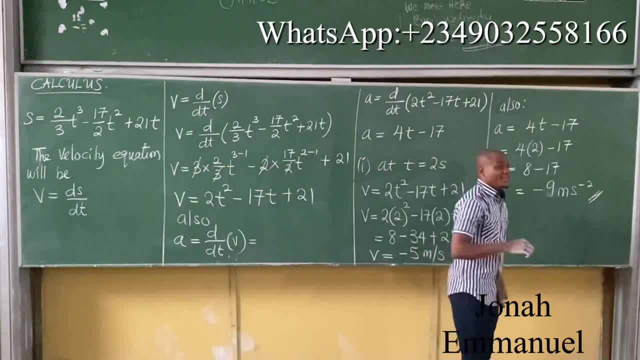 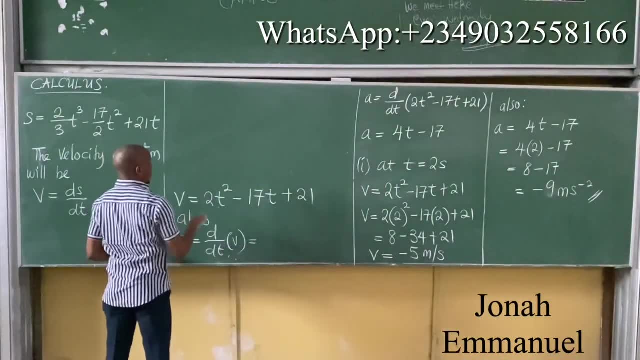 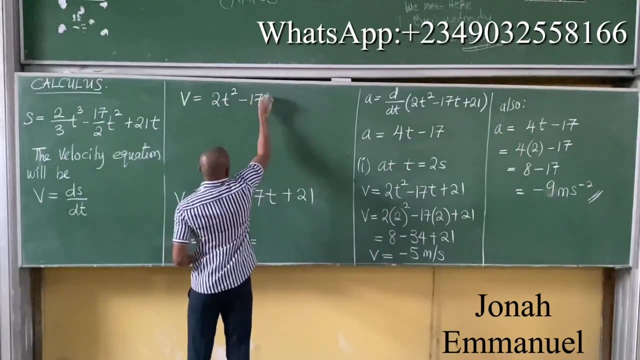 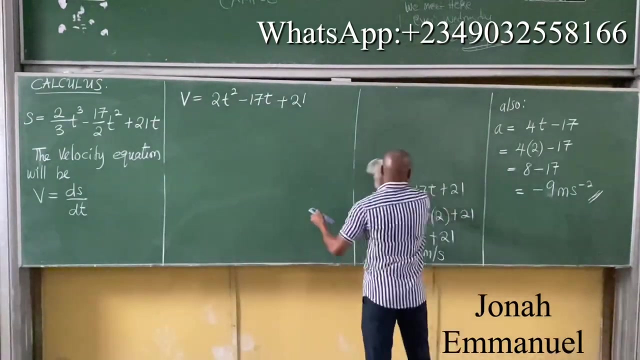 would be fun. when a body is at rest, its velocity is zero. so my equation is: V equal to 2T squared minus 17T plus 21. is that what we came up with? so we are here. we said if a body is at rest, its 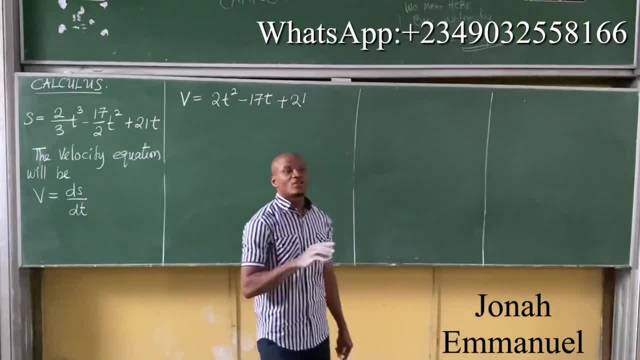 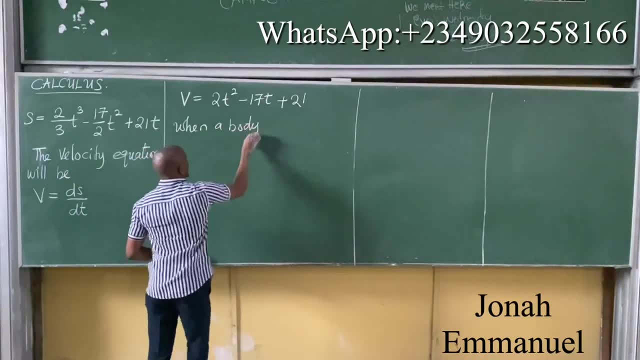 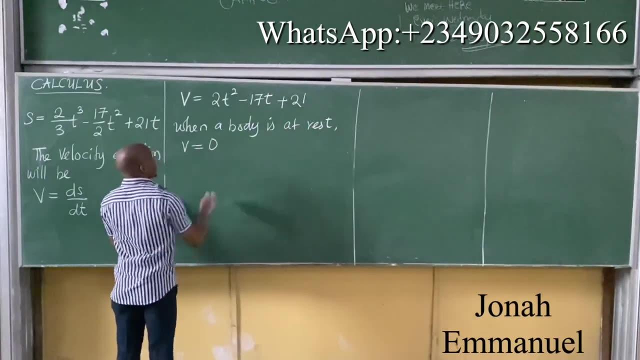 velocity is zero. look at this. so how do I solve that math? look at this. look at this. so how do I solve that math? look at this. so how do I solve that math? look at this. look at this. when a body is at rest, the condition is that V is equal to zero. so 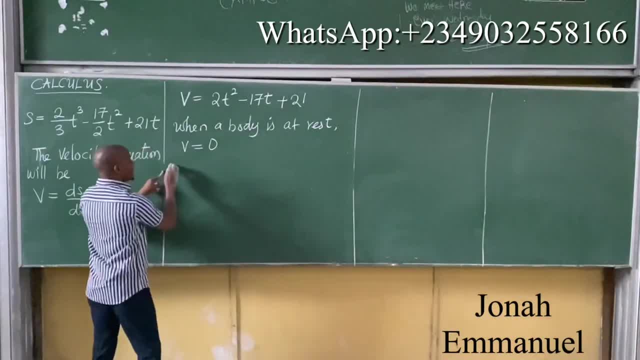 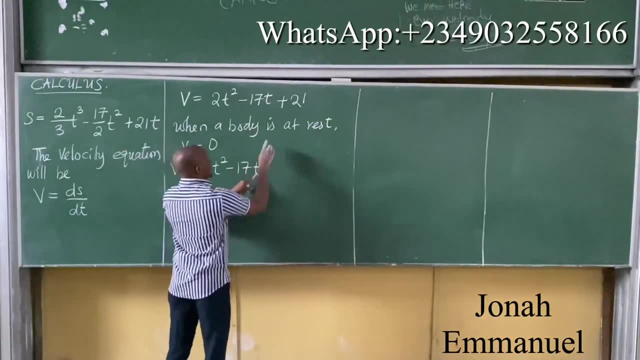 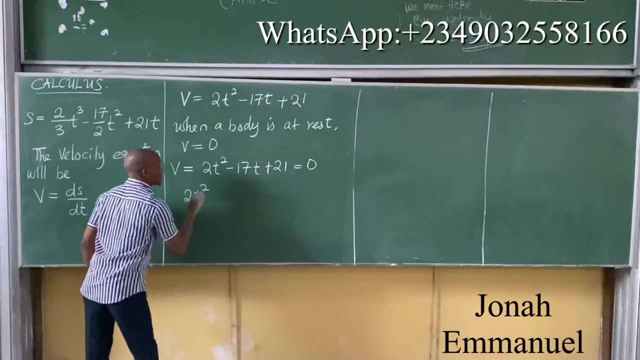 what next? I'll take my equation. but we said V is equal to this one. here: 2T squared minus 17T plus 21. we said this is equal to zero. I'll take this equation: that's 2, 2T squared minus 17T plus 21. I'll be equal to zero, please. what the equation is this? 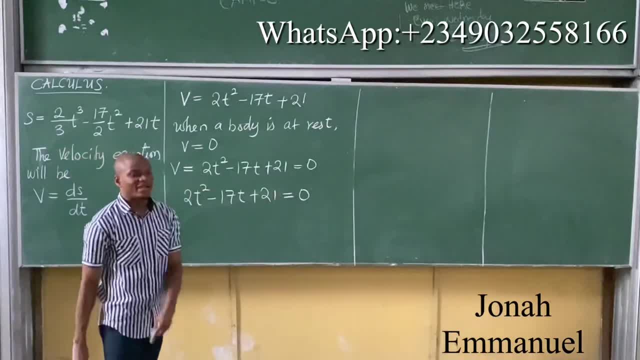 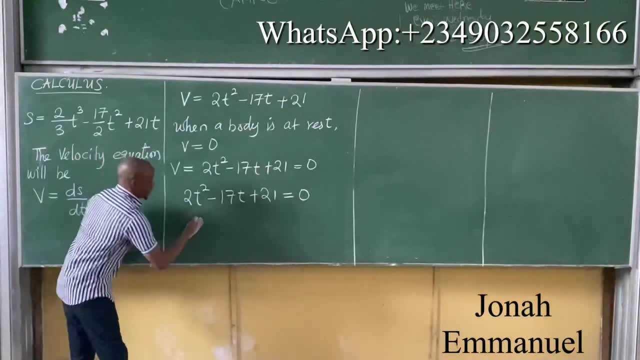 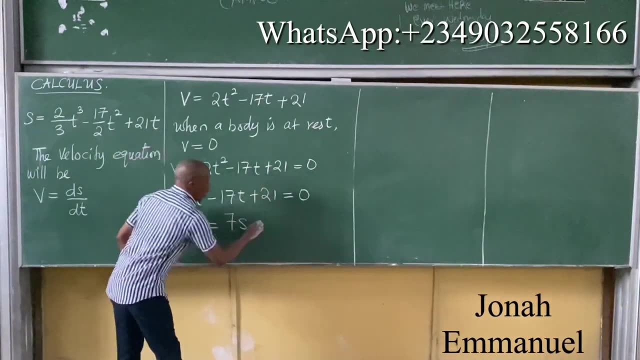 quadratic. please solve this one quadraticly. give me the answer, please. just for to calculator. please just give me the answer here. solve this one quadraticly. give me the answer here. solve this one quadraticly and give me the part of T. T is equal to what you get. 7 seconds is time, or what then? 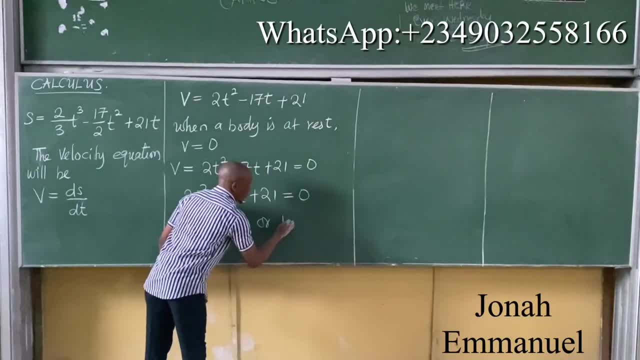 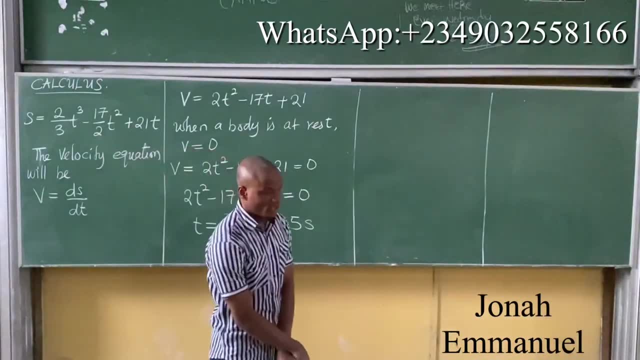 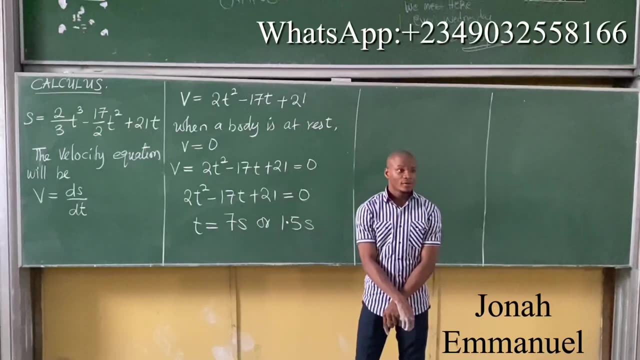 1.5. So t is equal to 7 seconds of 1.5.. Please turn 1.5.. Please turn, Is it correct? Please punch. A is 2.. A is what there Minus 17.. C is what. 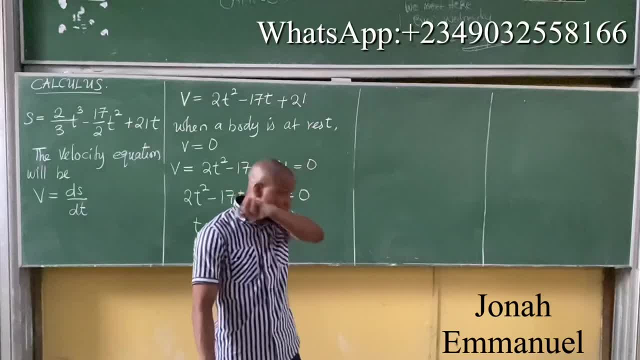 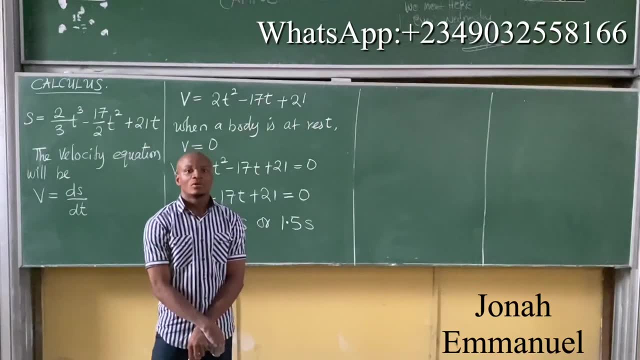 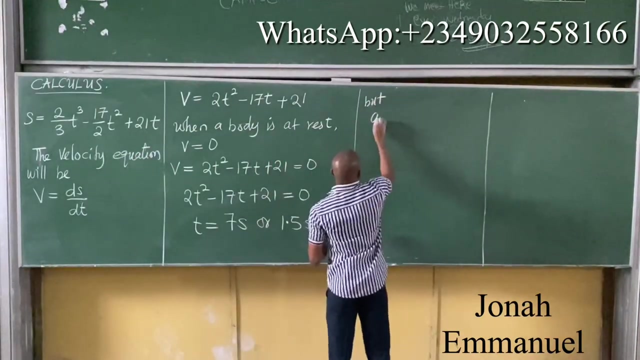 You get the answer. Alright, Now listen up, Look up this. You have to find what exactly. Huh, You have to find what there. Now listen, Listen. Give me your equation here, please. A is equal to what 40. 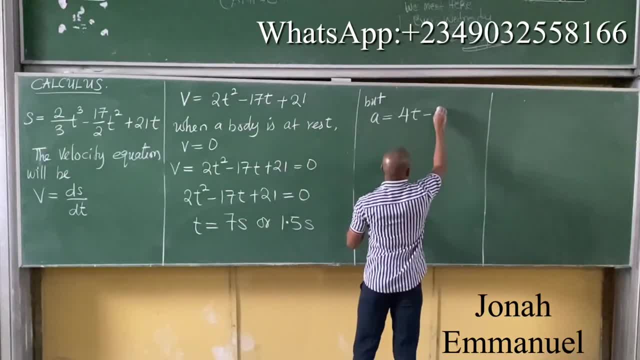 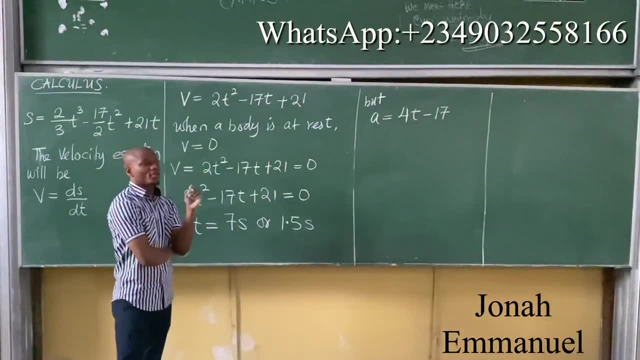 Minus what 17. This Listen When they say: find acceleration when the body is momentarily at rest. that means the velocity is there. From this equation, now solve it productically. At this point nobody is going to use any method convenient. You should have done this in first semester. 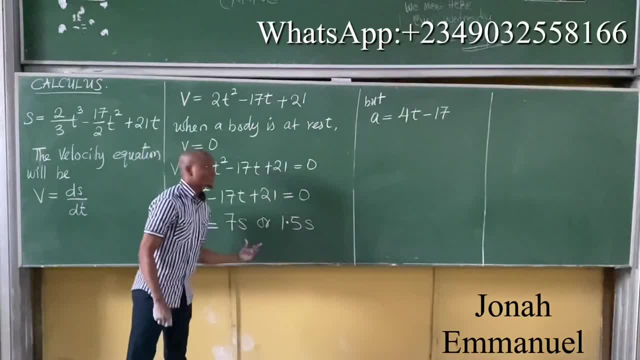 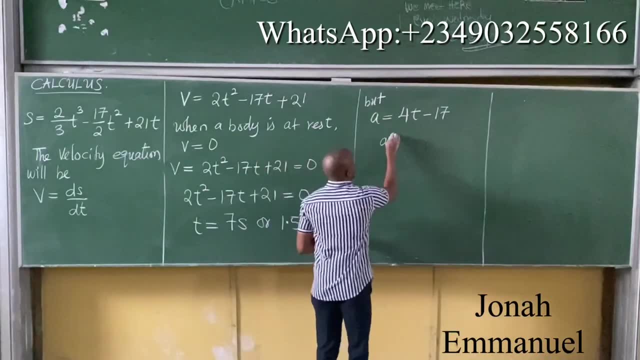 And you have these two answers Next up. put these two times into your acceleration. That's all. Put these two times into your acceleration. So first up you say at C, equal to the first answer there, 7 seconds. You have that A is equal to. 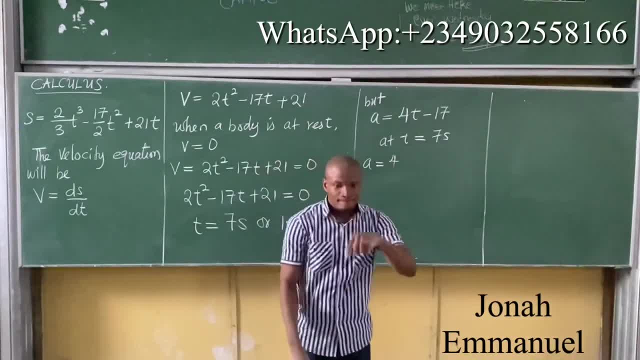 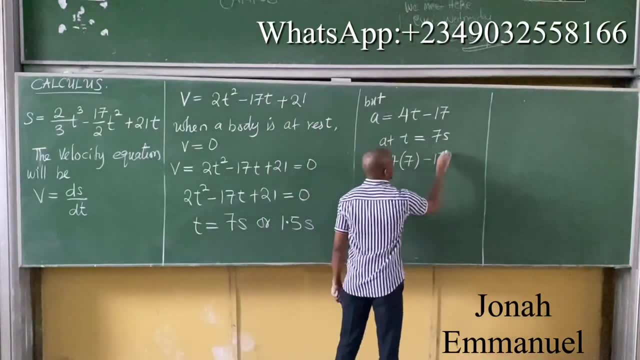 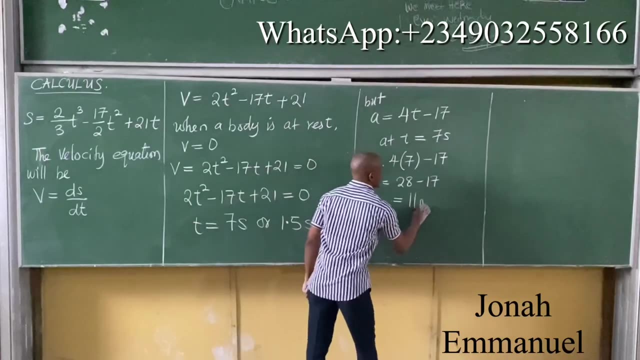 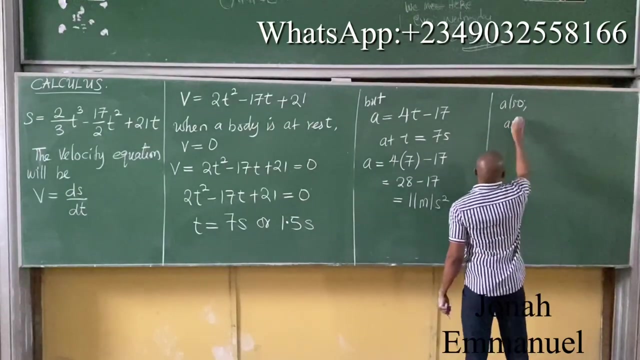 You have that. A is equal to 40.. What's T there? 7 minus 17.. What is that there? 28 minus 17.. That's what there? 11 meters per second, squared Also also also at C, equal to. 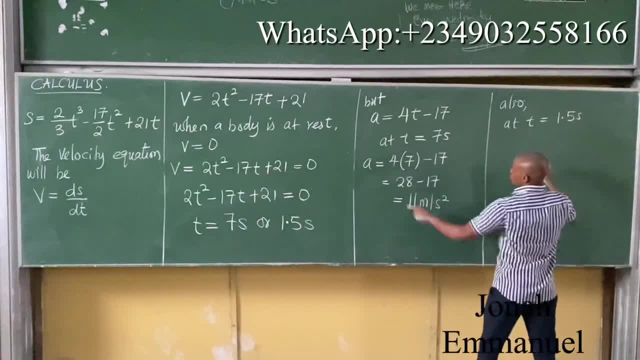 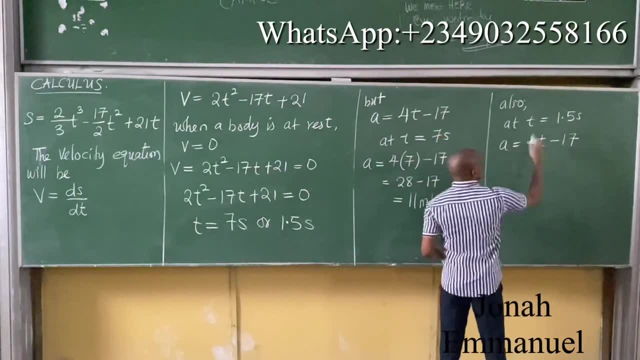 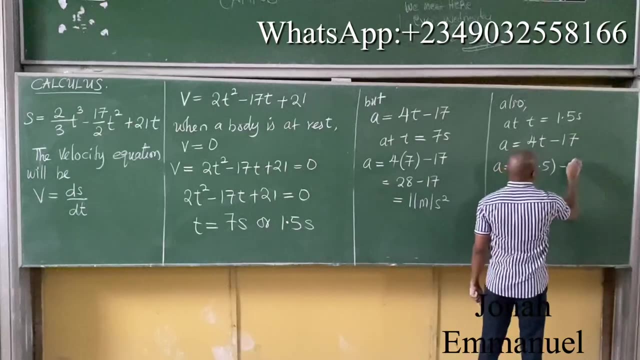 the second one here, 1.5 seconds. You have that A which is equal to 40 minus 17.. Which is at 1.5 A is equal to 4 into what I have here: 1.5 minus 17.. This gives you what there. 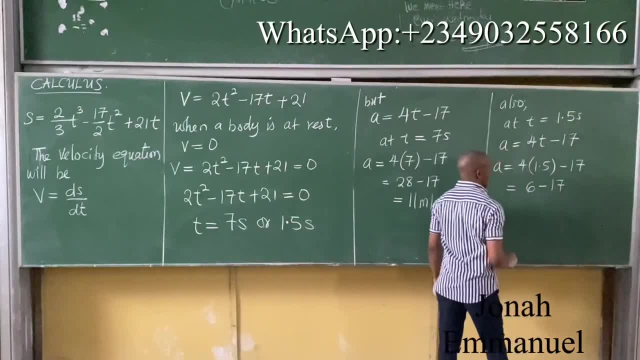 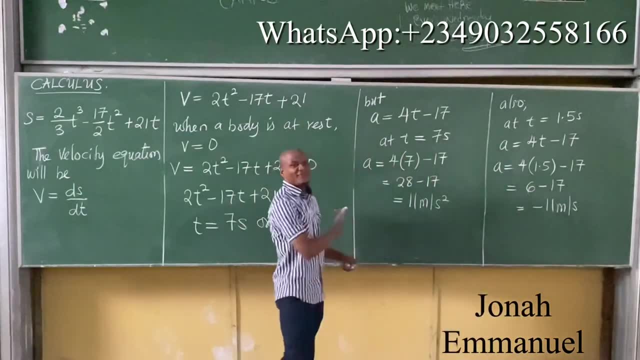 6 minus what there? 17.. Happy, What do you get here? 6 minus 11 meters per second. Now, what do you get? The same value, Happy, Yeah. But what there? Opposite what? This one here. 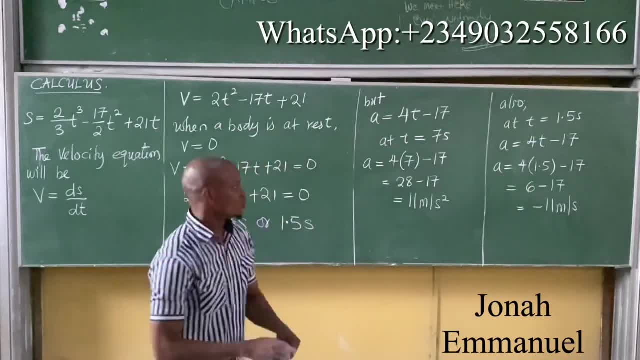 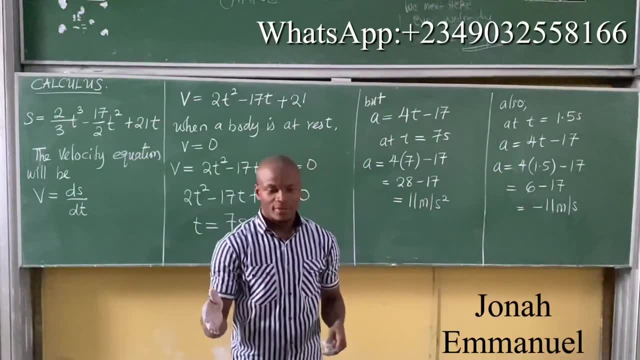 Which of them will be the actual one? Should it be this one or this one? Which of them? This one Should it be this one or this one? This one, Should it be this one or this one? This one, This one. 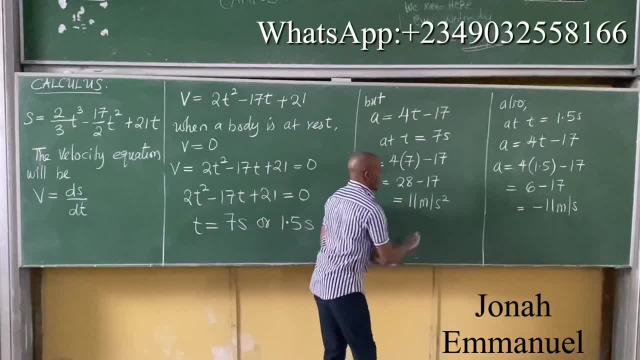 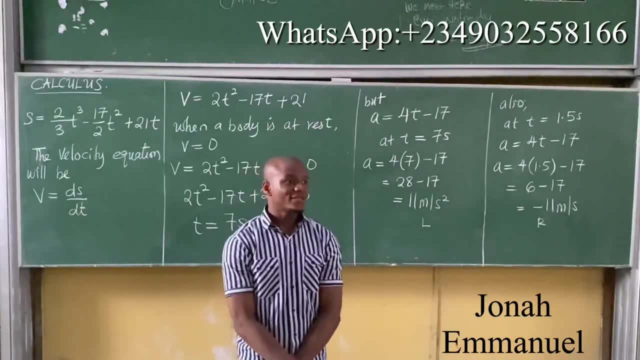 Should it be This A? Should it be left or right? Which of them This one? Which of them This one? Should it be left or the right Right? Left or right Right? Your original acceleration: was it positive or negative? 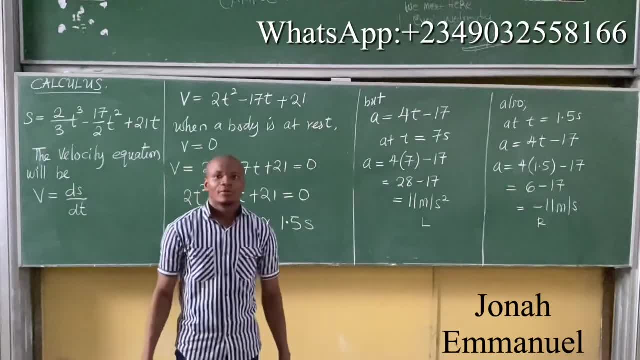 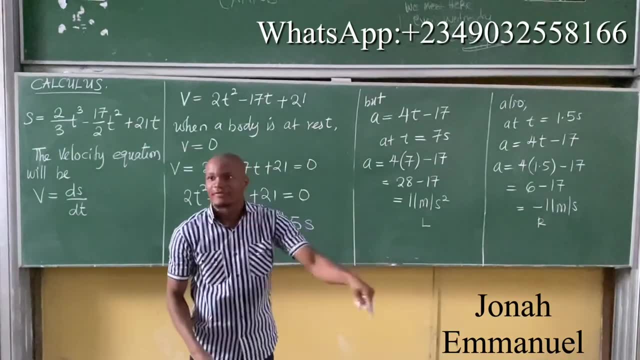 Negative, It has to be the right there. That's it. This one is not straight passing Right. You have to think about it. When you did original acceleration it was negative. So if you now have a negative and positive answer, negative there. 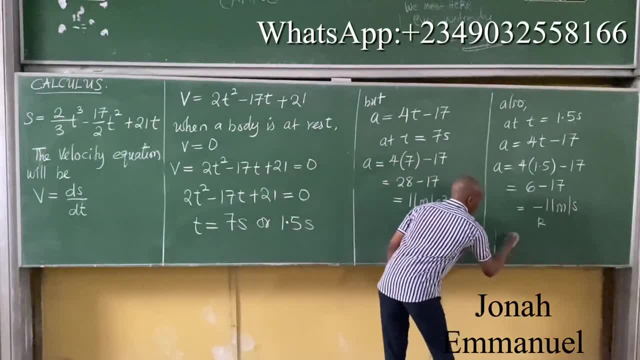 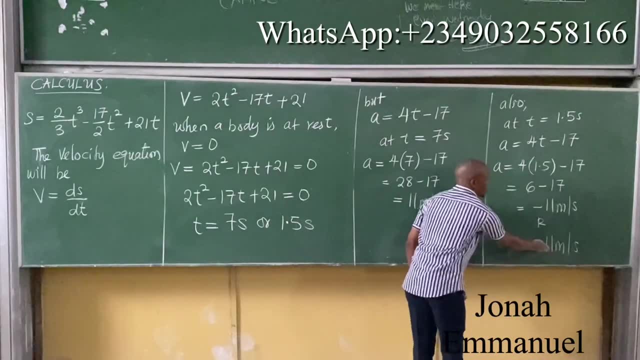 So any of them is correct. That means the acceleration is correct. It's equal to how big for this there, Minus 11 meters per second. I'll tell you what I'm giving you for that, Because when I did original acceleration I had a negative answer. 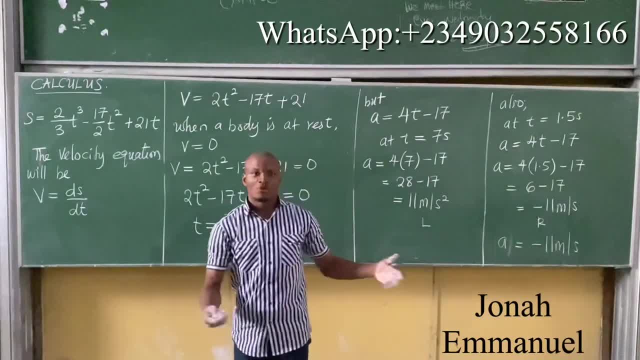 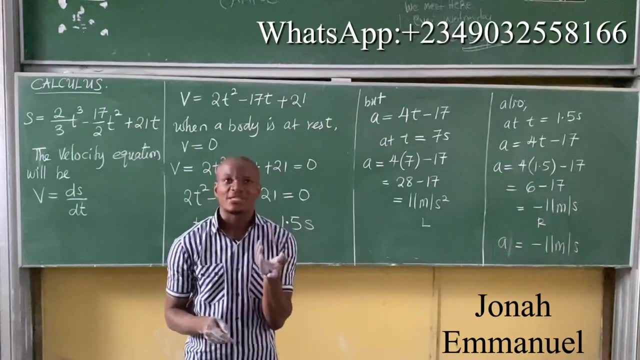 And since you know the things, I'll pick negative instead, For whichever way, It's still 11.. This is 11. So, when it comes to rectilinear motion, always note that when a body comes to rest, velocity is there. 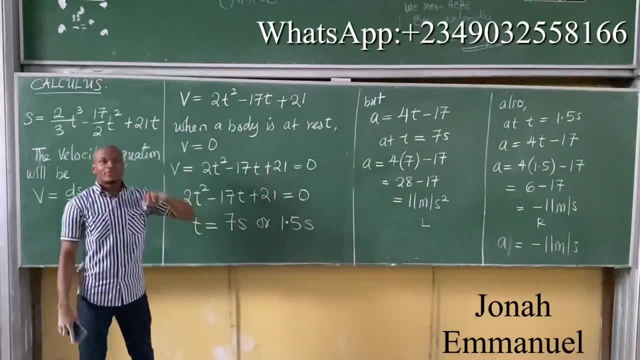 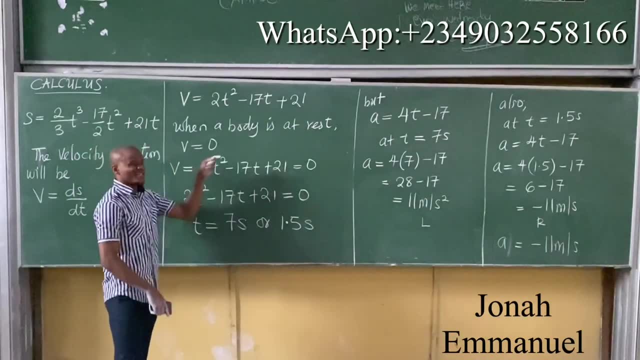 That's it All right. So I'm going to show you how to do that. Tell you what: Most times, sometimes at this point, when you have that dv, dt- sorry, ds, dt- which is V, is equal to zero. sometimes, when you get the value of V or the value of t from here, 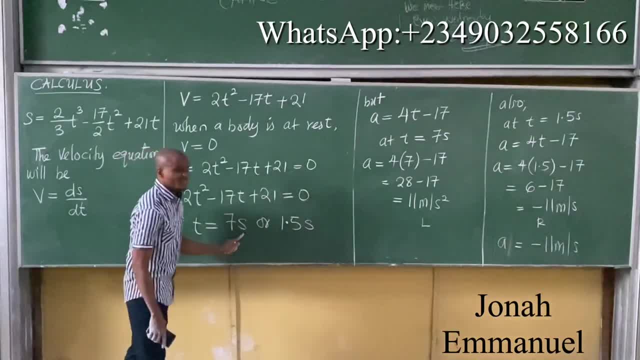 it will give you this answer as 1 positive and 1 negative. Listen up: When you solve this, it will give you this time as being 1 positive and 1 negative. In such cases, don't even bother with what there. 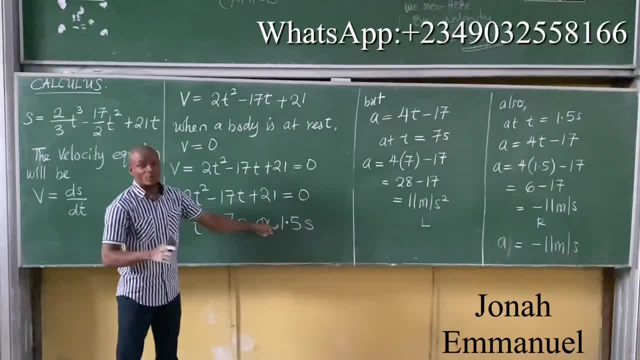 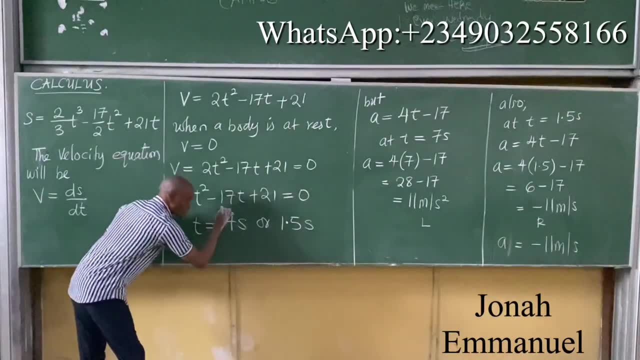 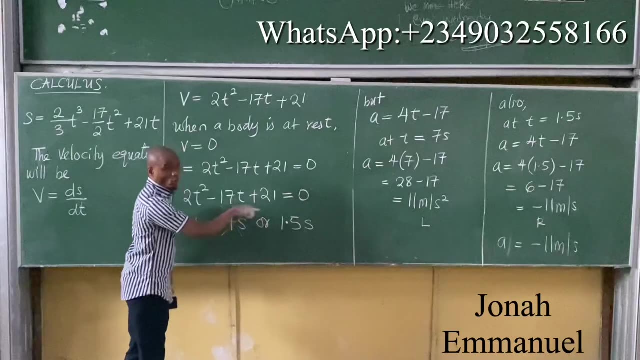 with what there Negative. Why Time cannot be negative. So let's assume my answer was, let's say, minus 7 and 1.5.. I will cancel this one totally. So you say, since time or t cannot be negative, hence it's equal to what there 1.5.. In this case, both of them are positive. 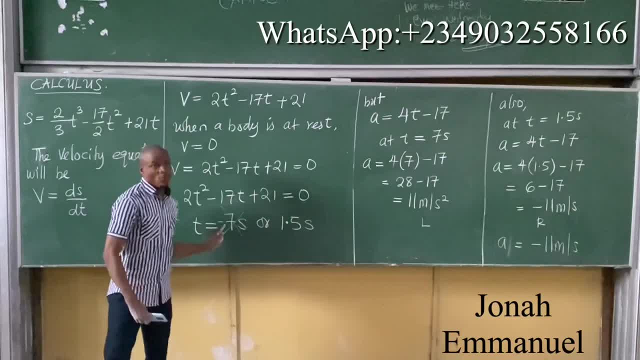 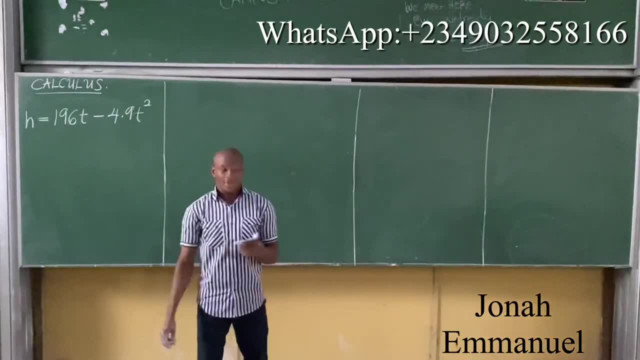 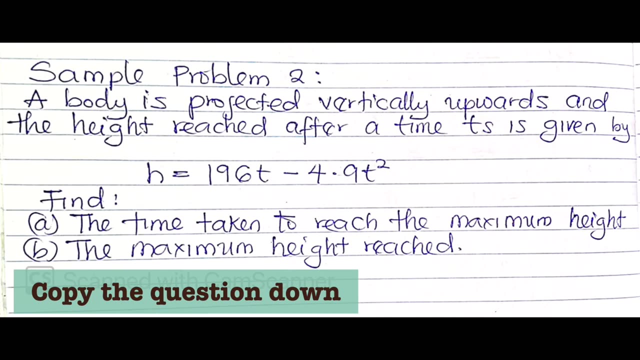 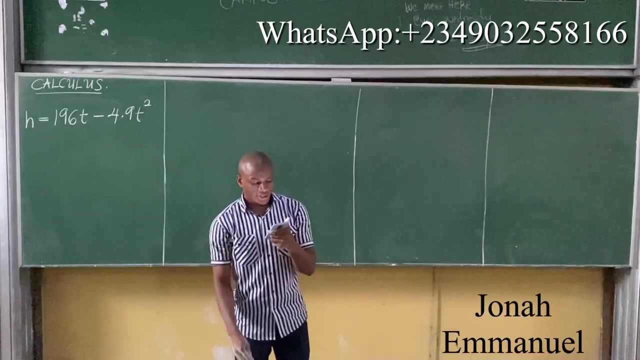 so I use both of them. But in the case where one is negative and one is positive, ignore the negative. Go along with what there Positive, All right. Question 2. A body is projected vertically upwards and the height reached after a time, t seconds. 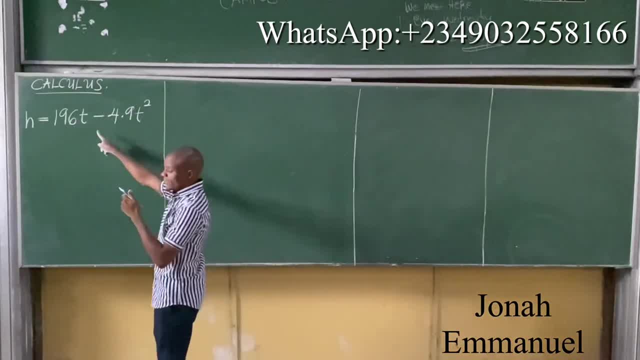 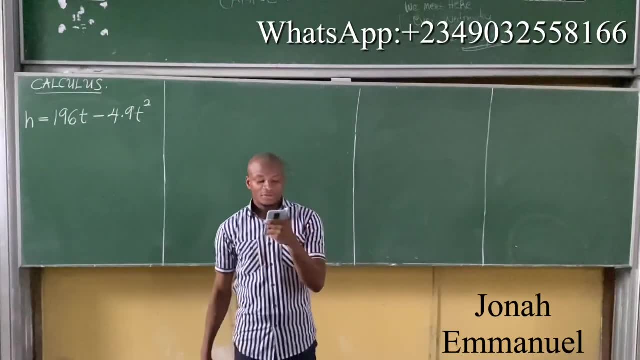 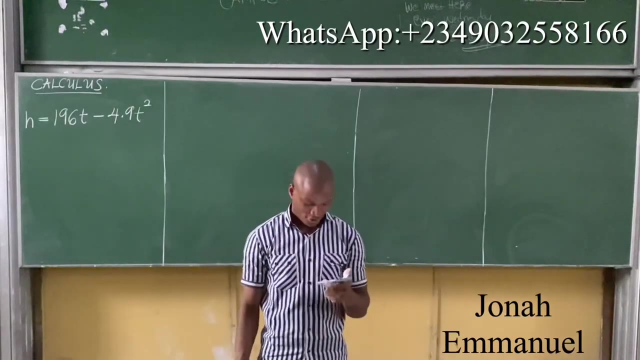 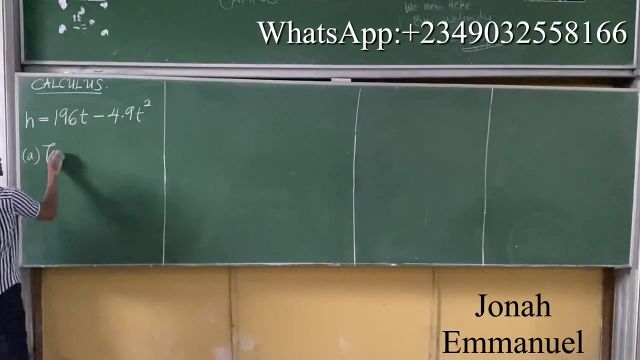 is given by h, equal to 192.. 4.6t minus 4.9t squared, Find A or I the time taken to reach the greatest height. I- I the greatest height reached. All right, Let's start with A Time taken to reach greatest. 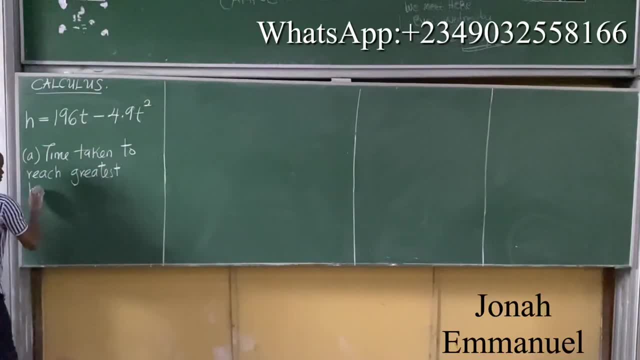 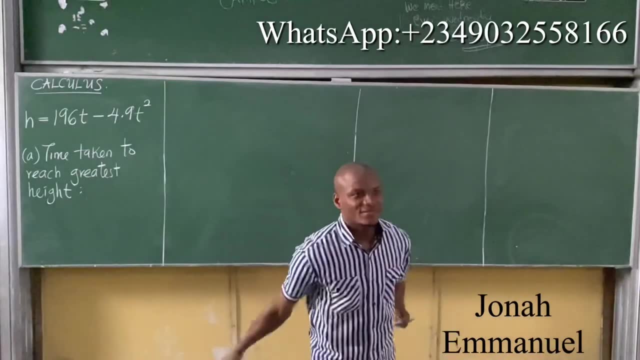 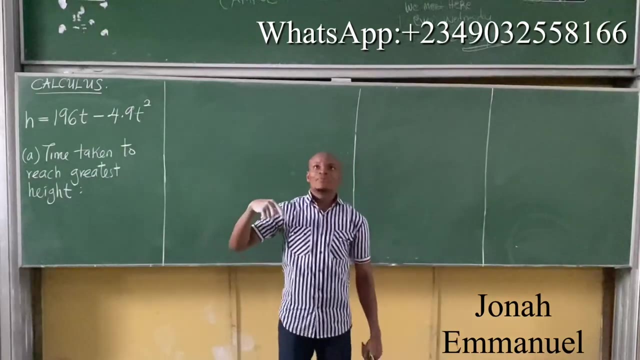 height, Please. my thesis is: when a body is at its greatest height, what's the condition of that body? Now hang on. In the previous example we said when a body is at rest, velocity, not acceleration Velocity, is zero When a body is reached the greatest height, if I 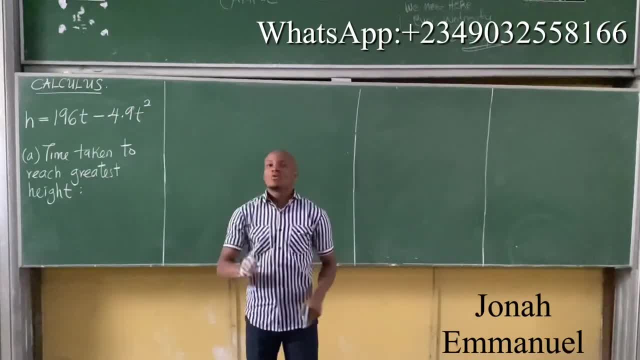 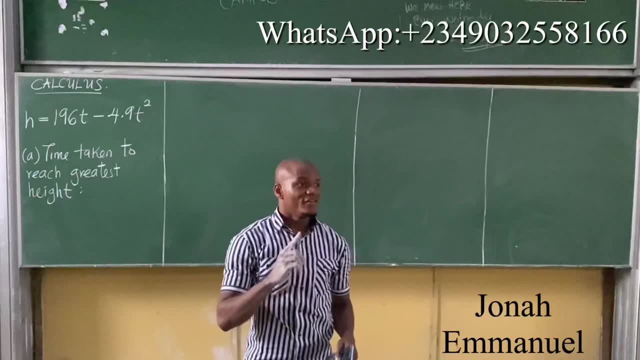 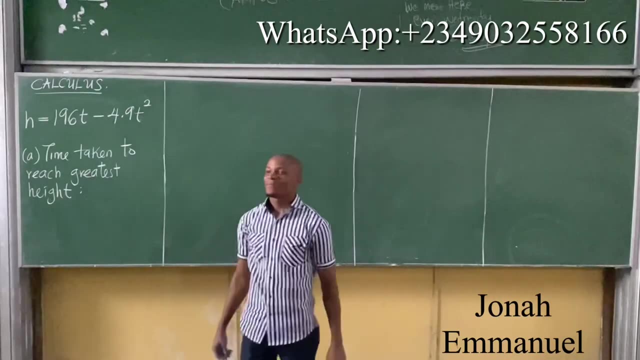 throw this chalk, I throw it up and it gets to greatest height. what's the condition? at greatest height, Velocity is zero. Velocity is zero. Yes, That's from free fall. I mean Yes, Right, Yes, Take that with you. At greatest height, the velocity is zero. Please note these conditions. 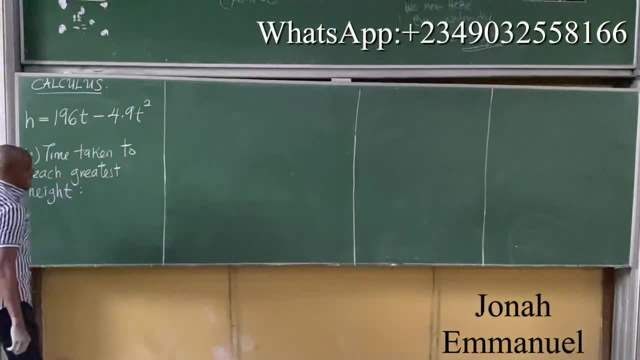 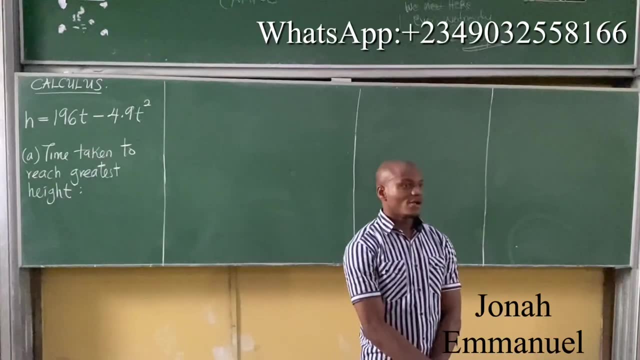 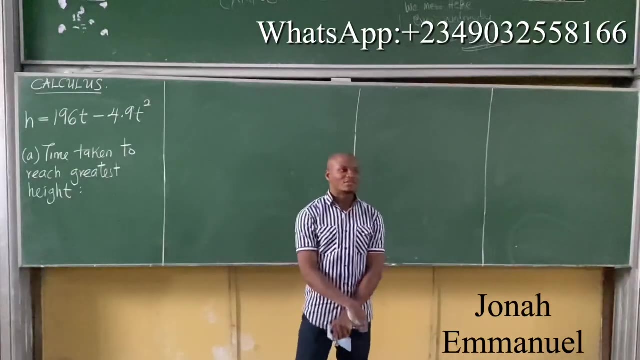 At greatest height velocity is zero. But I was giving height, not distance. So how do I get velocity from height? Huh, We said velocity is 2s over 2t, but I'm giving h or s. So how do I get the s over the t here? What do I do? 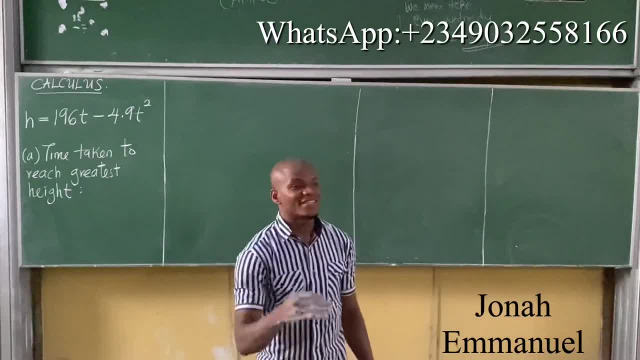 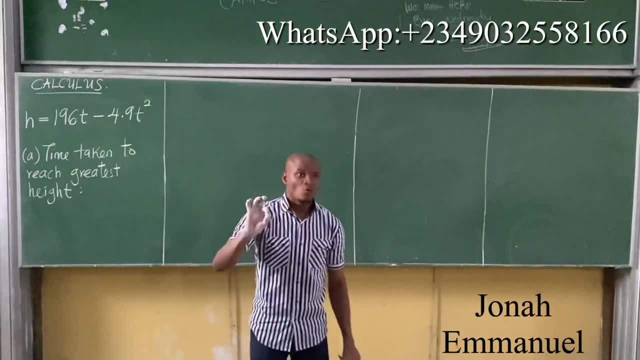 What does c? Listen? listen, Height is still distance. Difference between distance and height in physics is that when we say distance, we're talking about what there A vertical a, what Resultant motion. When we say height, look at this now. If I show this, it has gone a distance. 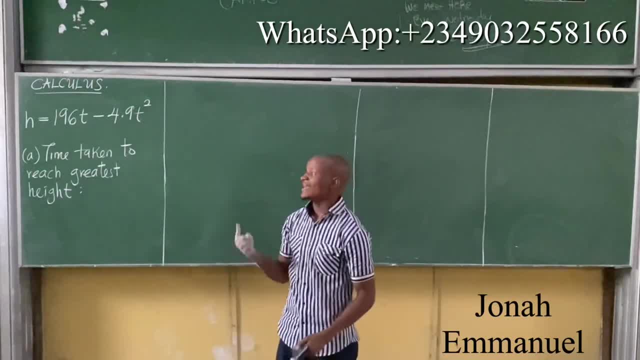 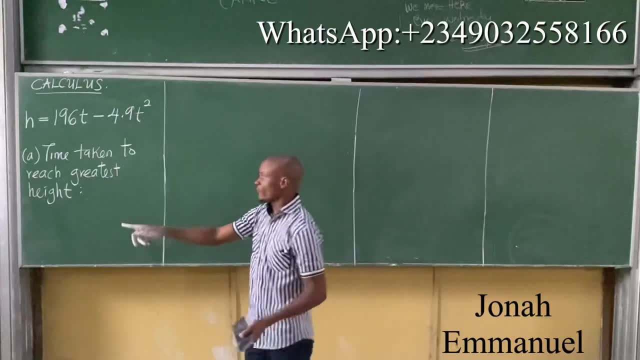 But this has now become what there, A height. So if I say height, what do I mean there? Vertical distance, So it's still distance. in what there, The vertical set, So it's still distance. So from here, condition is that v, which we know as the s over the t. 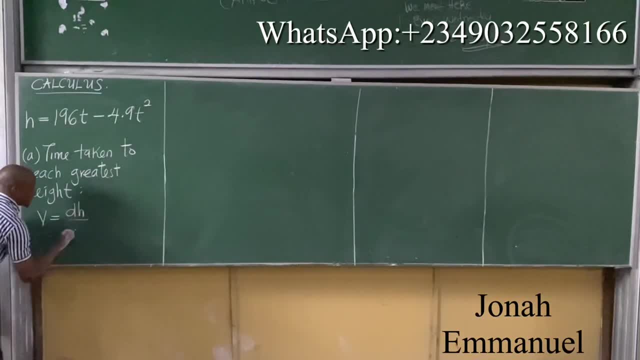 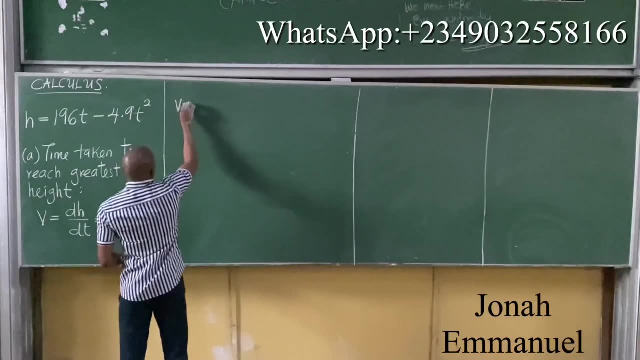 but in this case it's height. So because what there The h over the t is equal to what there Zero. That's the condition at maximum height. So I'll have that v which is equal to v over the t of h, And that's equal to z over the t of what h there. 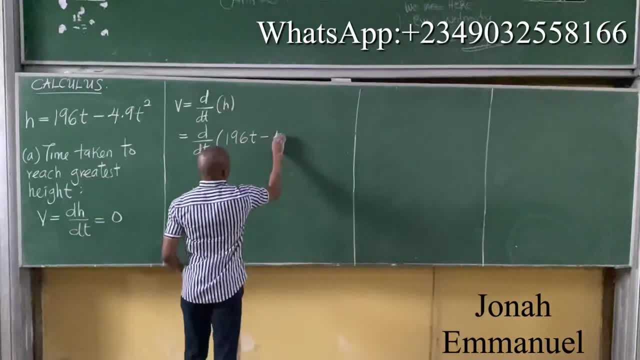 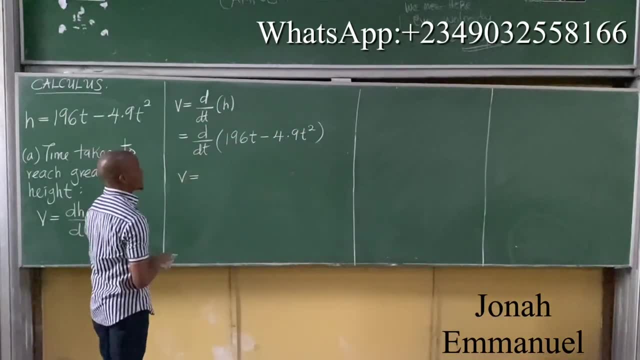 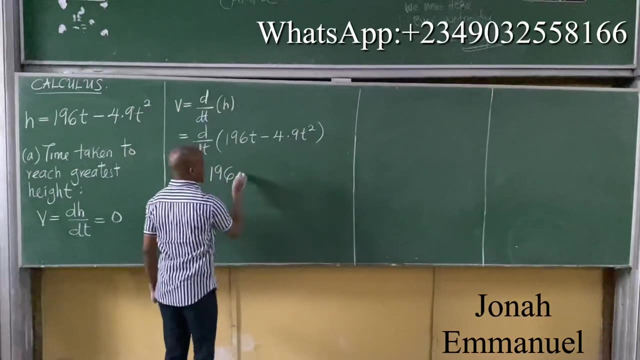 One, nine six, three minus four. point nine two. t squared, So v is equal to. I'll have to differentiate this: What do you all get? Differentiate this, What do you get there? One nine six. Differentiate this: What do you get there? 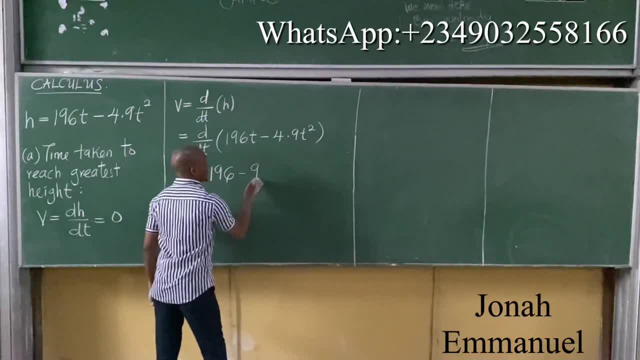 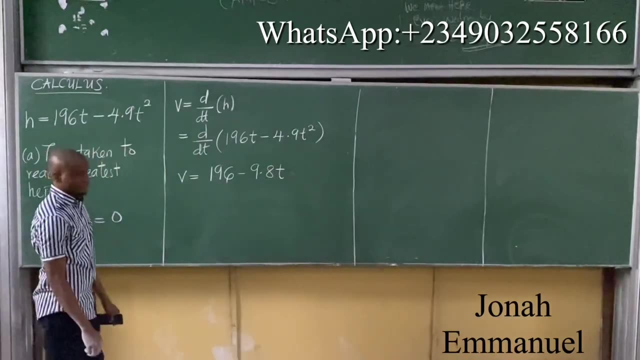 Two times this a v. That gives what there? Nine point eight, See a v. Yeah, Two times this one gives you nine point eight. Of course, two minus one is what This is just what's it called general method of precision. 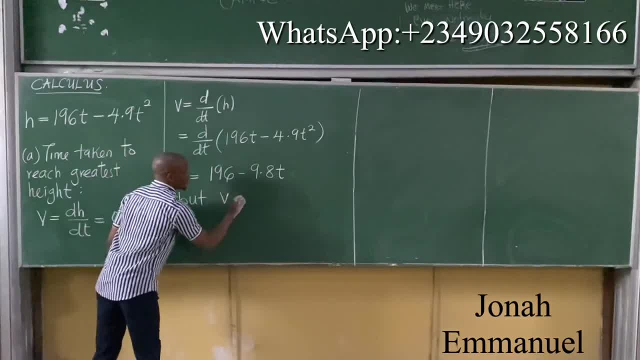 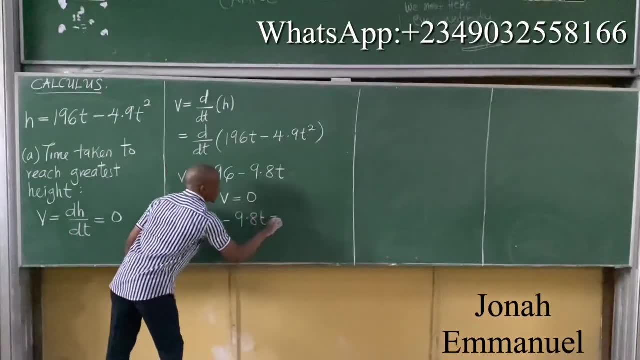 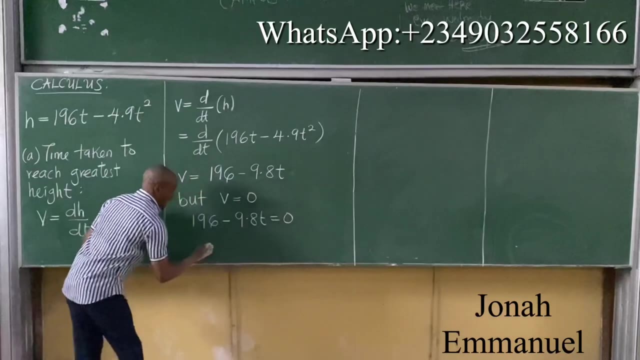 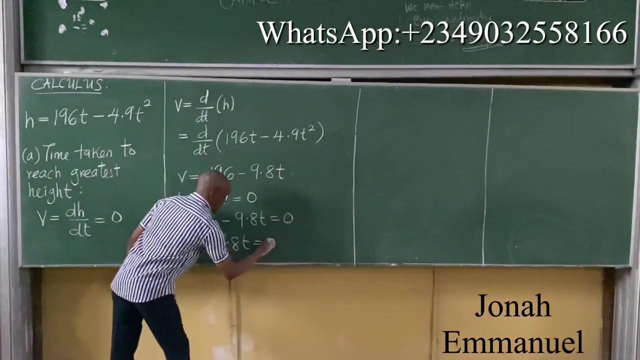 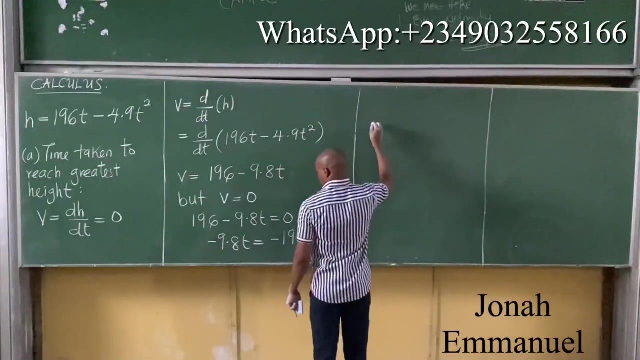 So it's said that v at beta size v is equal to zero. That means this: one nine six minus nine point eight, t is equal to zero. Make t subject of the formula- I'll move this man over here- So I have minus 9.8T is equal to. here it's positive. constant becomes what? there Negative, 1, 9, 6.. So get T. T is equal to, here it's positive. now constant becomes negative. Here it's D negative. 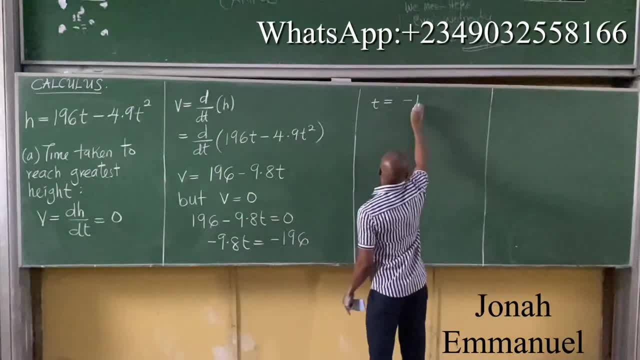 So T is equal to divide both sides minus 1,, 9,, 6, all over. divide that by this minus 9.8.. Minus times minus T is equal to what there? Sorry, 20 seconds. 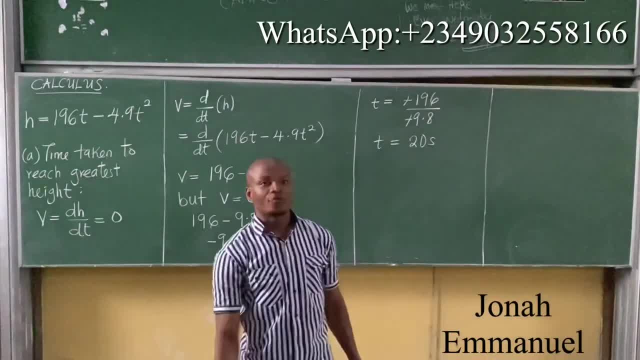 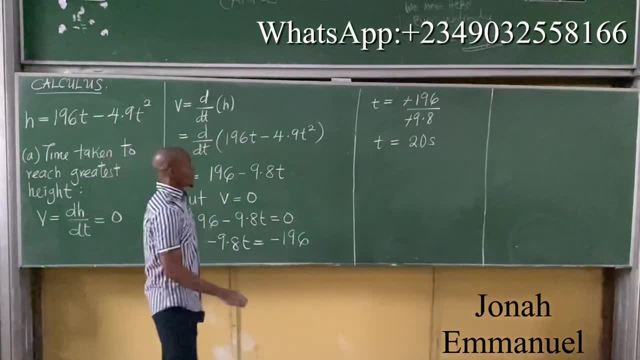 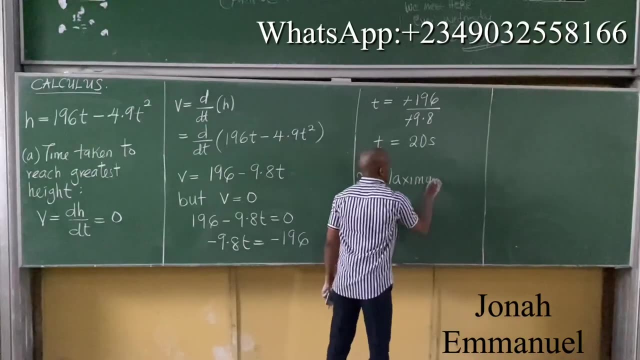 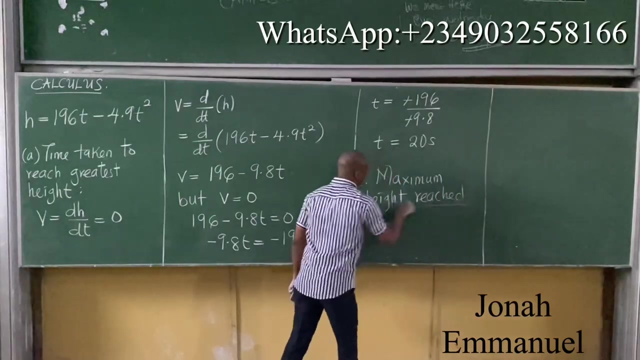 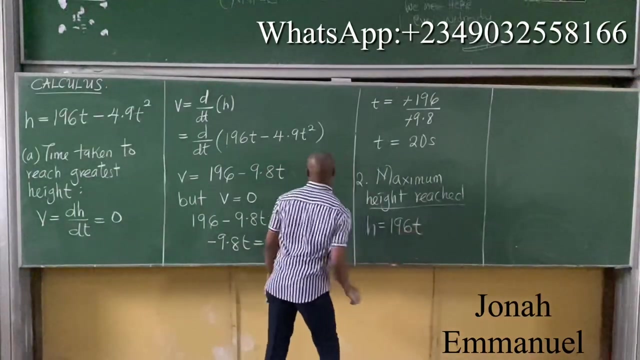 So number 1, find the time taken to reach maximum height. It takes 20 seconds for that body to reach maximum height. Number 2 says: find the maximum height, Maximum height reached. Maximum height reached. Alright, so H is equal to 1,, 9, 6T minus 4.9T squared. 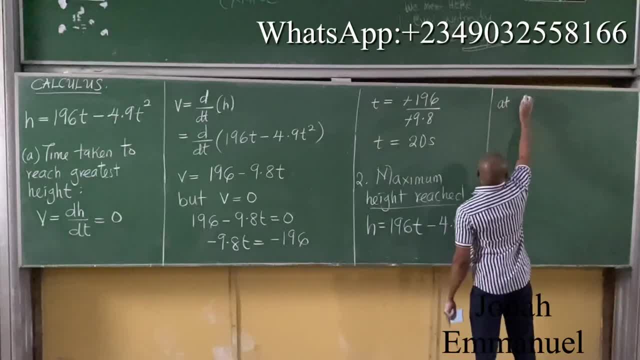 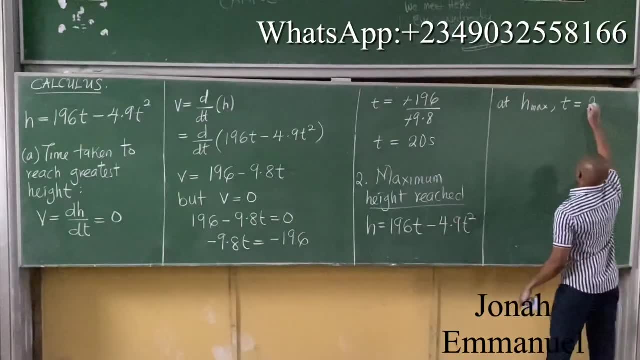 We said at maximum height, that's at H max. At maximum height, that is time. T, It's equal to 20 seconds. It takes 20 seconds to reach maximum height. So what do I do here? It's as simple as putting the value of T into the H equation. 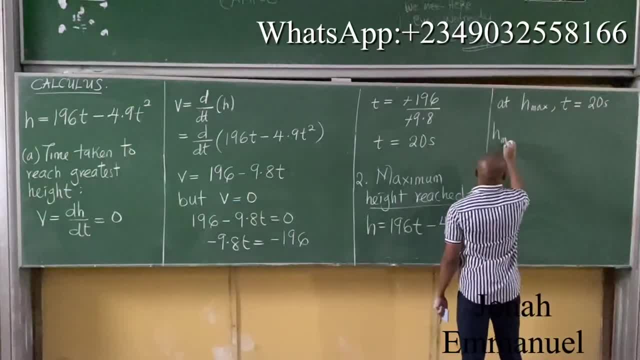 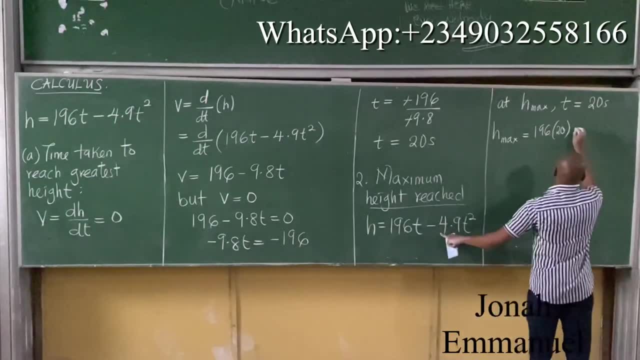 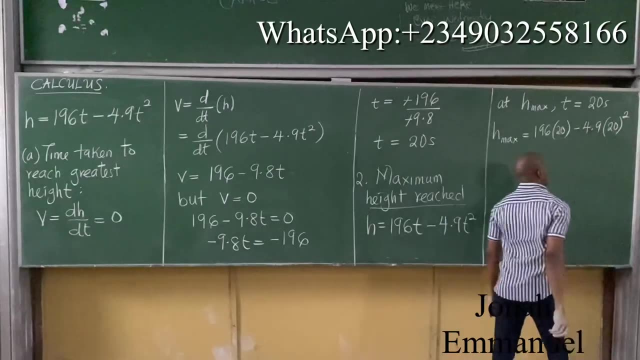 So I will now be having H max. H max is equal to 1, 9, 6 into 20, minus 4.9 into 20.. That's T. It's a square, So 20 squared This will be equal to. 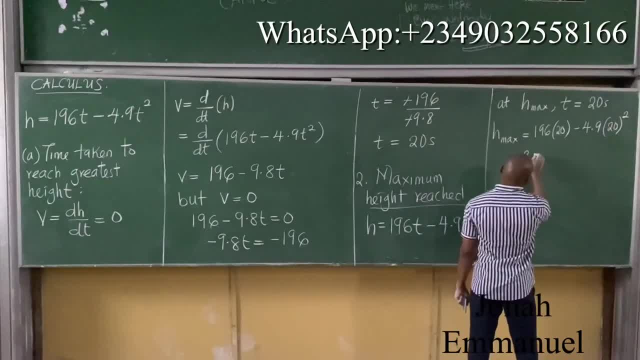 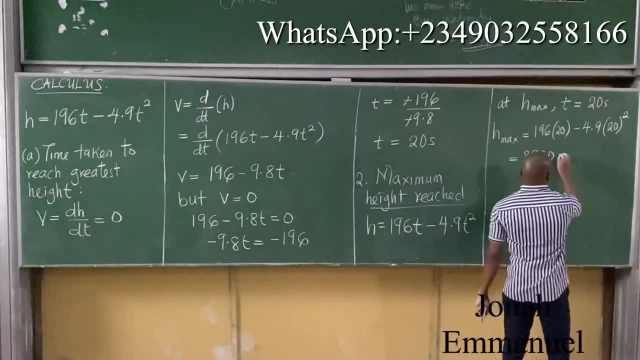 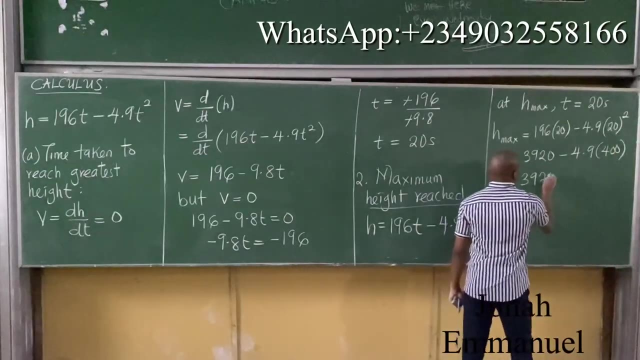 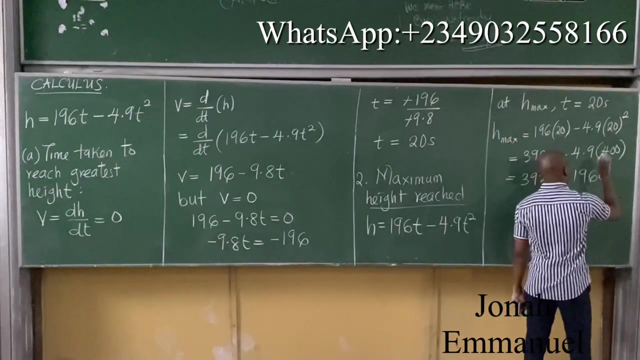 It's equal to 3, 9, 2, 0,. yeah, minus 4.9 into 400, that's equal to 3, 9, 2, 0 minus 6, 3, 12, 1, 9, 6, 0, right: 1, 9, 6, 0.. 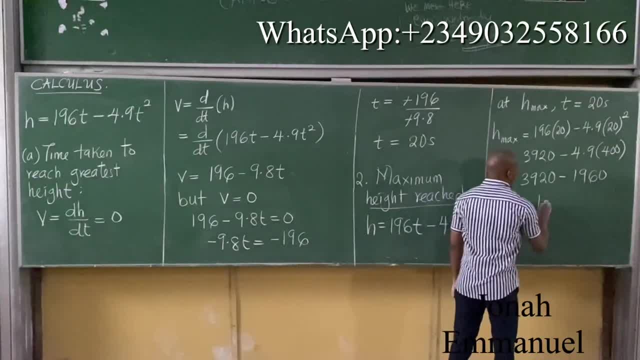 Subtract this. What do you guys get? 1, 9, 6, 0.. 1, 9, 6, 0. again 1, 9, 6, 0.. 1, 9, 6, 0. 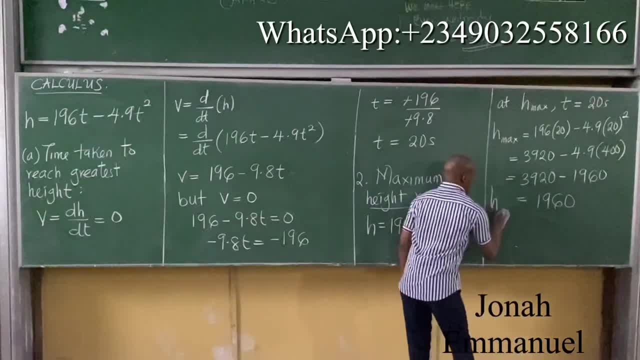 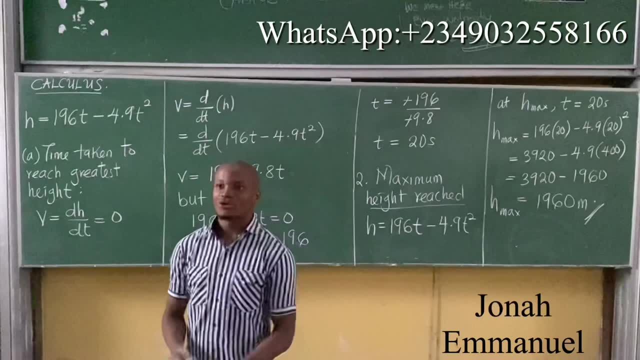 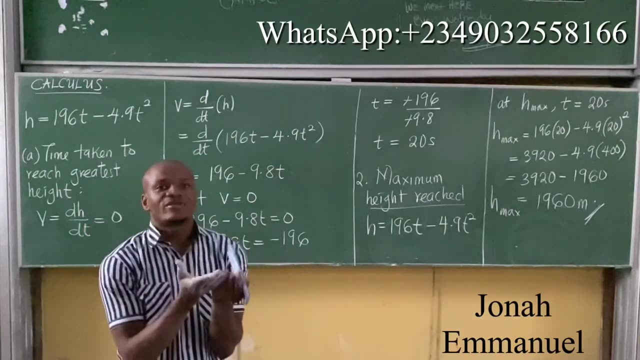 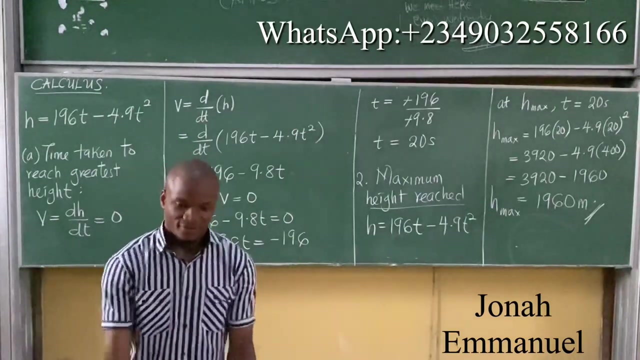 Alright, Units, please, Units, please, Meters. That recalls the maximum height. So the key to solving these problems hinge on: can you translate the question into numerical sense? At maximum height, At maximum height, V zero. One is at rest, V zero, and that's it.